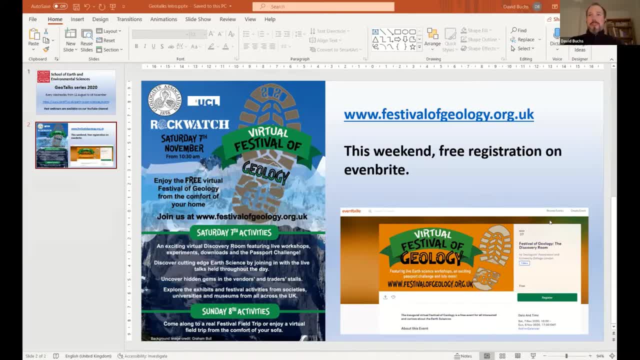 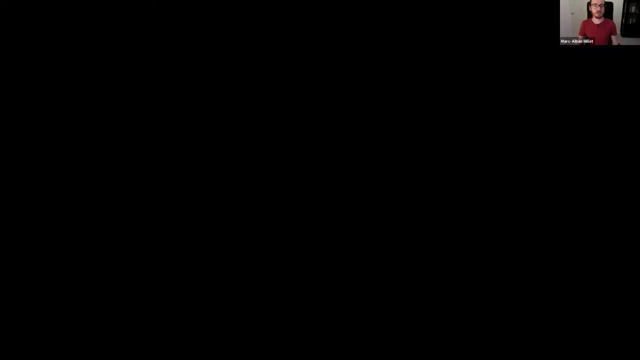 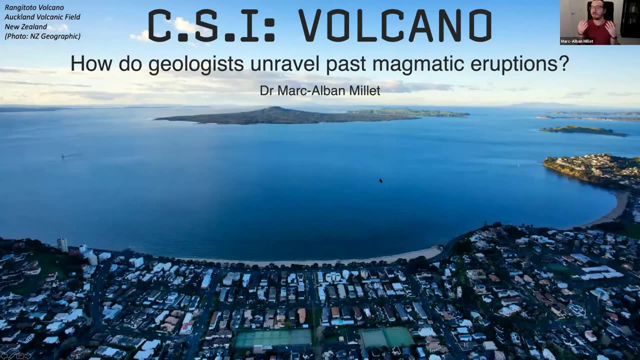 I think now you could share the screen with us and you could start your presentation. Okay, thanks very much, David. Yes, that should be now, and this okay. so I think you should be all be able to see now. so, yes, today I'm going to talk to you about. 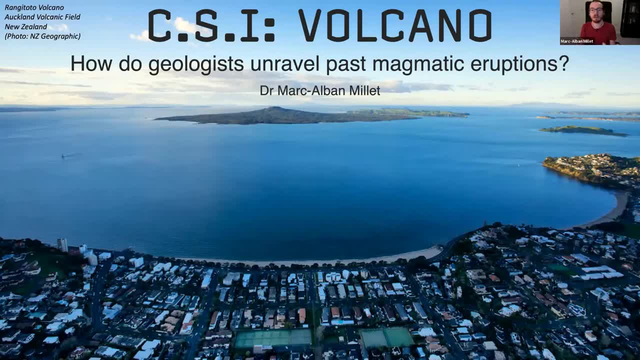 how geologists can actually study past volcanic eruptions, and this is obviously a major concern in terms of risk and hazards in some populated areas and you know, there are many places in which that we don't have historical records and we still need to know what happens, because they 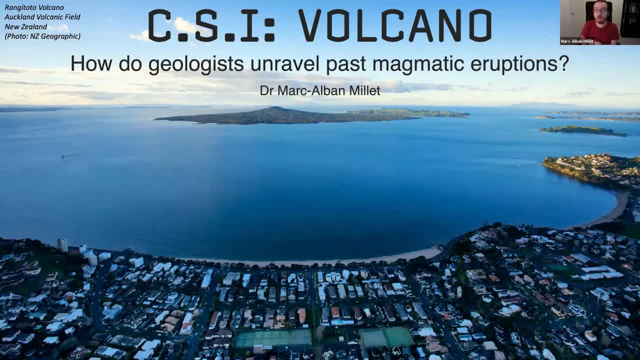 might carry significant risk to the local populations. Here is an example here in my title site of the city of Auckland- okay with this- in actually quite sizable volcano here which is called Rangitoto. Auckland is the biggest city in New Zealand. it's about one and a half to two million. 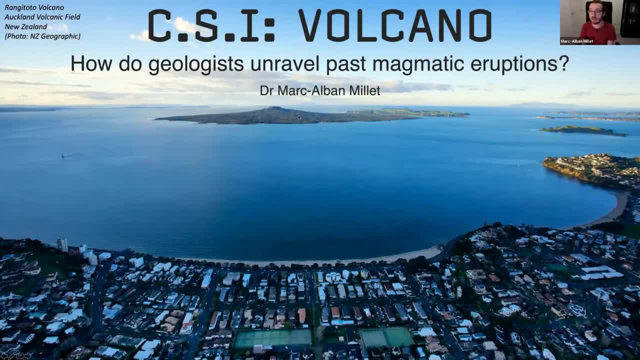 people, and this volcano here is only about 700 years old, okay, so you could imagine that if such an eruption could occur right in Auckland harbour right now, the city would actually be in big trouble and there would be massive- you know- human and economic damage. So I think it's important to 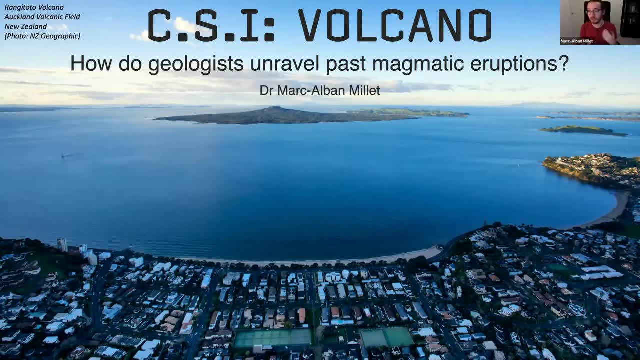 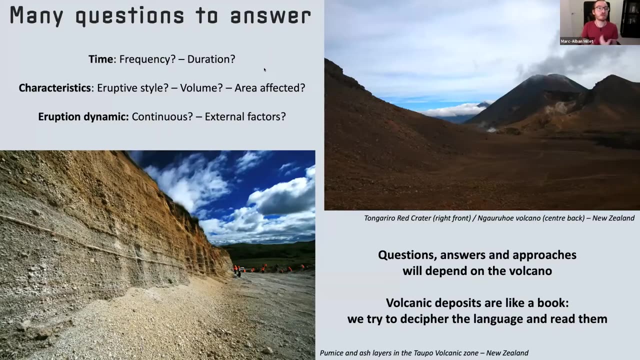 be aware of that. okay, so this is really the reason why we do this work. is you know? so how? what's the role that geologists and how can geologists help in in doing this, this work? okay, because there's many questions in here and maybe the first one is actually time, okay. 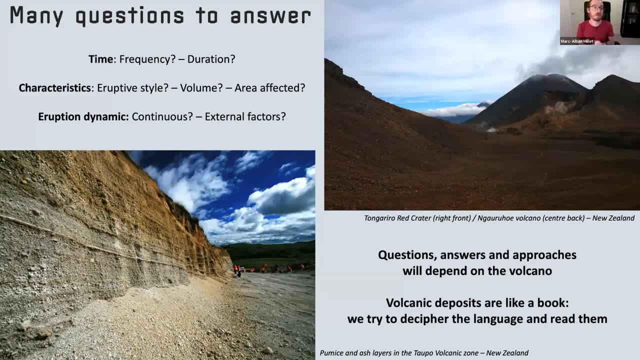 how often does this volcano erupt? okay, a specific volcano erupt. what's the frequency and how long? for what was the duration of that eruption? okay, what can we expect? and all of the things to do, for example, what was that eruption? and basically what this is trying to basically. 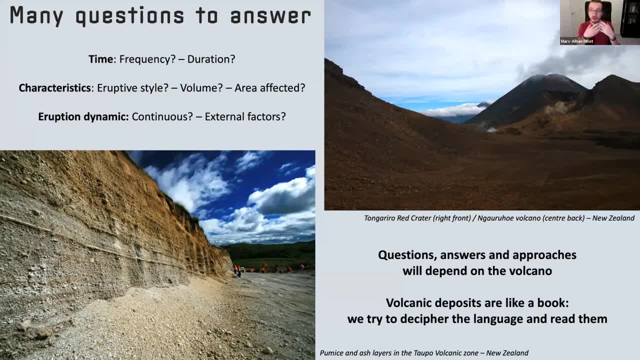 understand the behavior of any specific volcano. what were the characteristics of these eruptions in terms of eruptive time? was the lava just erupting calmly and slowly and just you know, going down the flanks of the of the volcano, or was it actually an explosive eruption? okay, which? 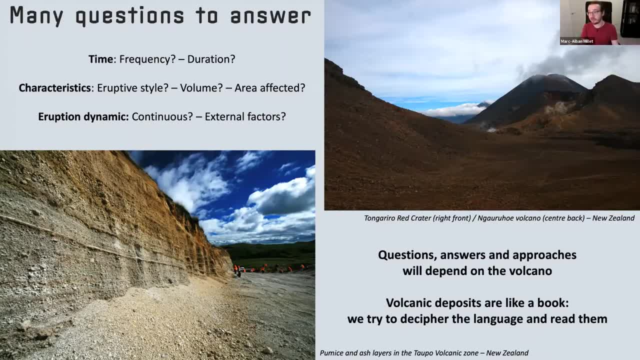 which would be much more dangerous. for example, what was the kind of volume that we can expect and the area affected as well? okay, would need to look at eruption dynamics. What is continuous? Was it stop and start and sort of jittery? And so the questions and answers and approaches are going to be different from every. 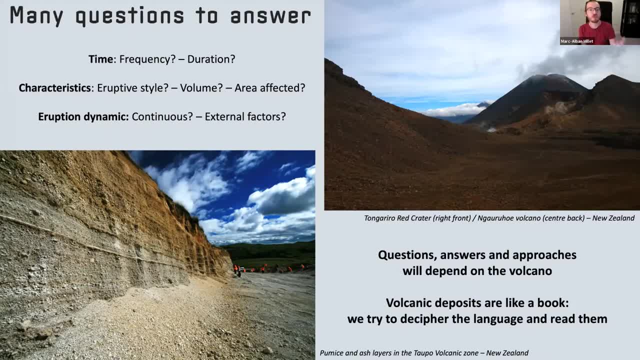 volcano that you're going to look at. You cannot simply use the same method over and over again and blanket out every volcano on Earth. That would be too easy. However, there are some common threads, And one of the things that I'm going to highlight to you today is actually detailed. 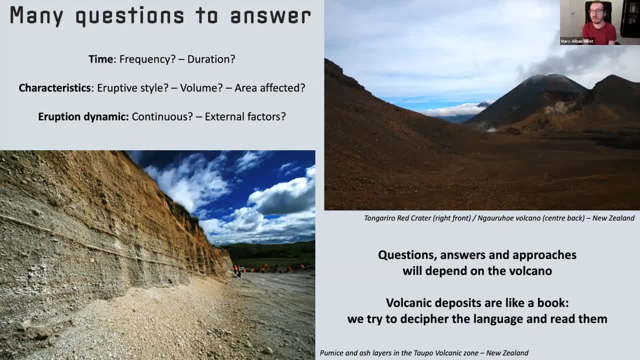 petrographic and geochemical work on key archives and key components of volcanic eruptions, so either the glass shells or the crystals themselves, and how we can use novel technology in chemistry laboratories to actually say a lot of things about these questions here. So volcanic deposits: they look like a book, They are like a book. We just need to find. 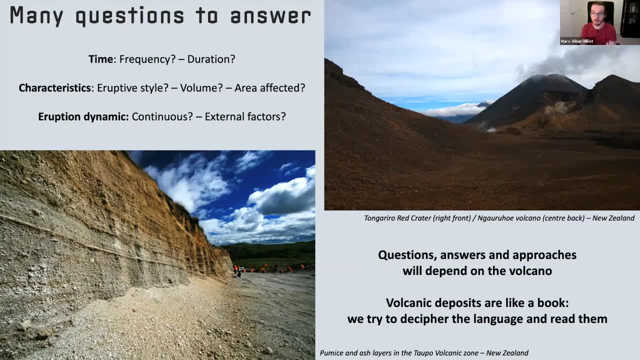 a cause to decipher them, How to be able to learn, how to read them. So in here I can see two good examples. On the bottom left here these are permission ash layers from the type of volcanic zone in New Zealand which I've got to work on and I will present some stuff at the end of this talk on. 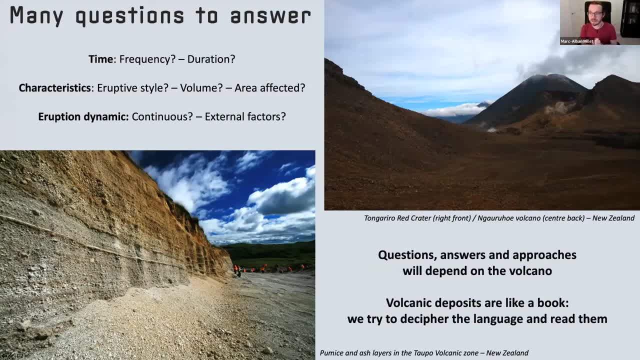 And these are actually students here nicely wearing their high-vis vests, working on it on a field trip that I used to lead when I was living in Wellington And in here. this is another highlight of New Zealand. This is the Tangariro Red Crater in the Tangariro Volcanic Zone in. 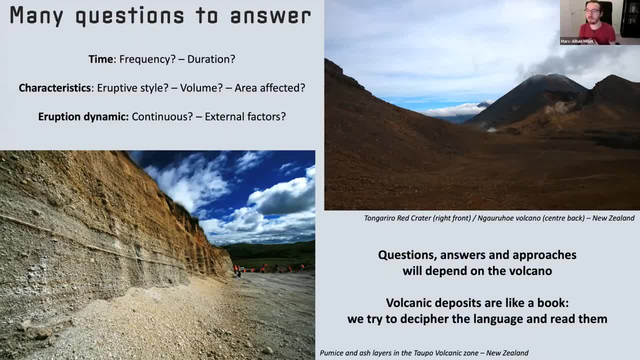 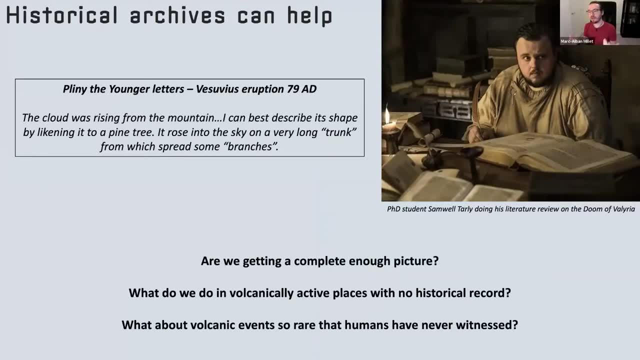 New Zealand as well. So both of these are different types of eruptive deposits and both of them needs to be understood correctly. So quite often, actually, historical archives will be able to help, And we know this because the first volcanologist ever was Pina Younger, who was just this person that actually started. 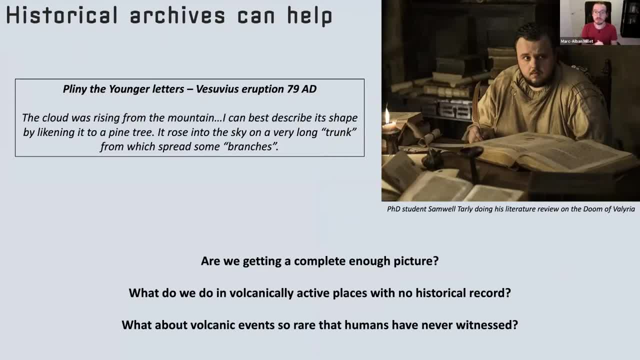 to describe the eruption of a volcano And the first artist to describe the eruption of a volcano of Vesuvius, you know, in 79 AD, the one that destroyed the city of Pompeii, and he actually just started describing what was happening. And you know, this is, these are. you know, there are. 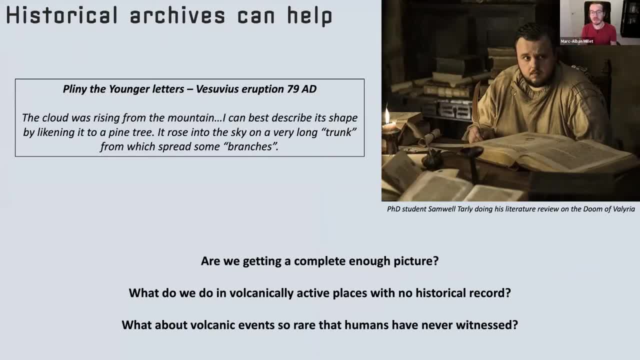 many records like this in history, over history. these are absolutely essential, but that doesn't beg the question, you know, are these, I know, are these records giving us a complete enough picture of what happened? and also, what do we do in volcanically active places where there are no? 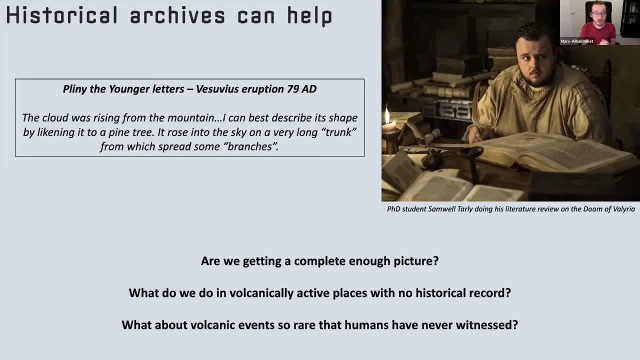 historical records whatsoever. We still need to understand these And also that also implies that we can only study volcanic eruptions through these kind of records on volcanoes that act on human timescales but not actually volcanoes actually work on these kind of timescales. We do know. 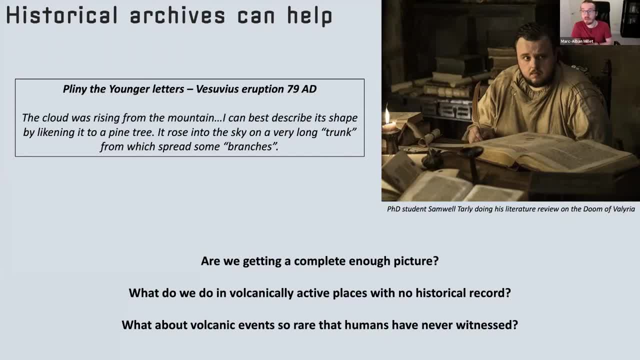 that there are volcanic events that are actually huge, extremely rare and so rare that humans actually have never witnessed them, And here I'm talking specifically about super eruptions. and this will be the second half of this talk, Okay, so in here I'm going to mainly 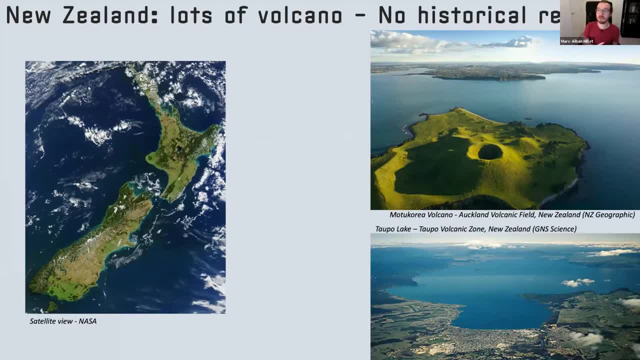 talk about New Zealand volcanic activity here, and that's because this is a place that's very close to my heart. I used to live there and work on these volcanoes, and I'm going to take two specific examples here. The first one is what we call the Auckland volcanic fields. okay, which is? 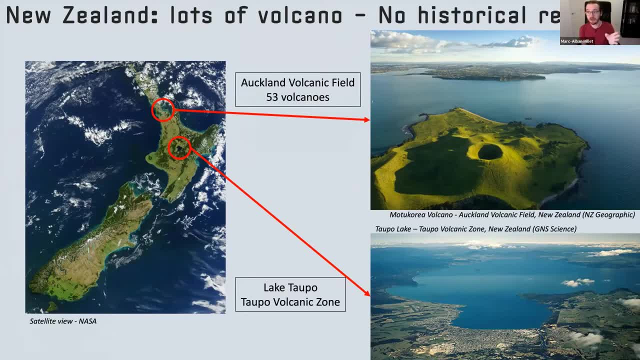 composed of 53 volcanoes that were that are erupted, present within the city itself, okay, and the latest one erupted about 700 years ago. so we know it is an active field. we just don't know when it's going to erupt next, And because you have a city of one and a half million people in there, there's 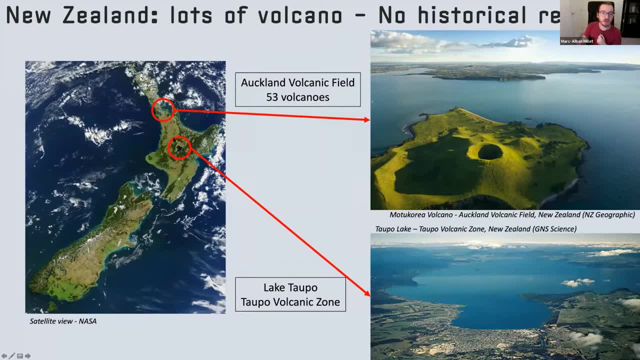 huge risks involved here. And the second one is Lake Tampo in the Tampo volcanic zone- okay, which is here in the IAL photo from GNS Science- And Lake Tampo is a completely different beast. This is the youngest super eruption super volcano on Earth. This, this specifically. 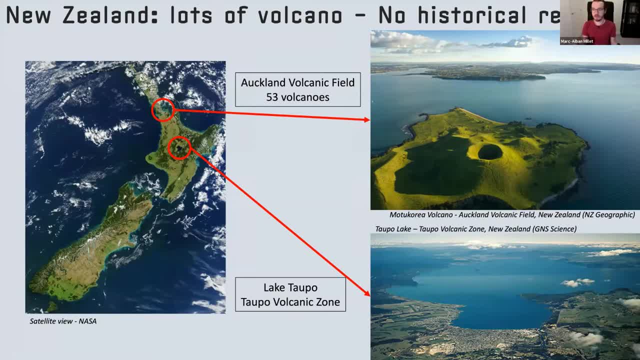 Lake creates momentous volcanic eruptions- and I'm going to detail that a bit later in this talk- and the youngest one of them is occurred about 24,000 years ago- okay, the you know- with some of the eruptions basically being, you know, 300,000 years ago or so, or even a million years. 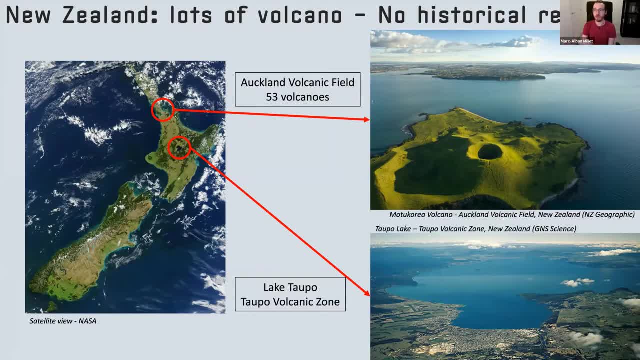 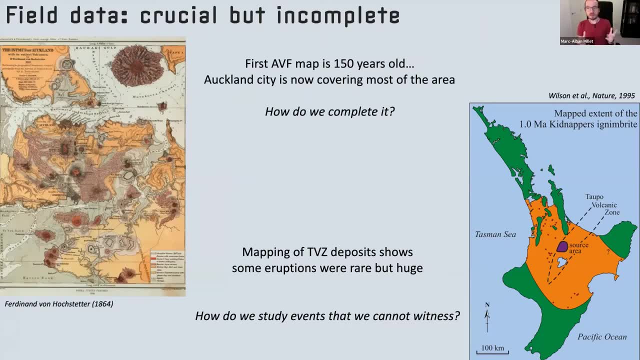 ago. So we know this is going to happen again, we just don't know when. okay, So how about you know both cases? the first thing we'll need to do as geologists is field data, and field data is absolutely crucial. Okay, we cannot do our work as geologists on these kind of deposits, on these. 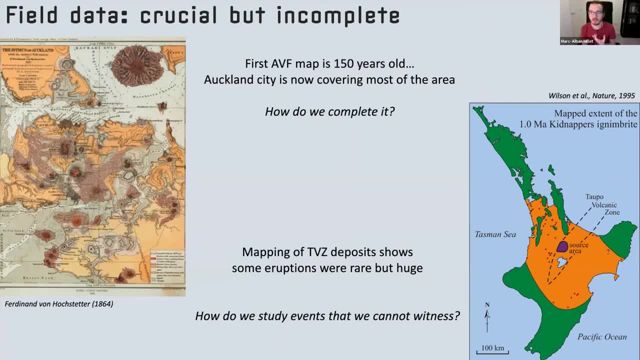 kind of questions if we do not have a good record of what the field data is. So the first Oakland volcanic field, or ABF, is actually about 150 years old. Okay, Oakland City is now covering most of the area, so we know we need to complete it, but we don't know how because actually, since it's built, 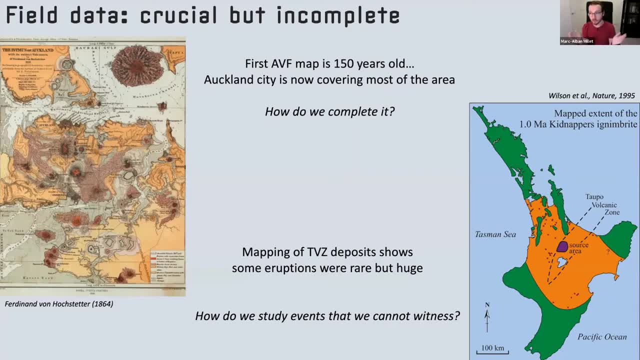 over these volcanoes. sometimes they've been quarried over, just being bulldozed over, and we sort of. we need to understand where they are now and and how they formed. okay, i stress as well that you know, when talking about historical records, new zealand doesn't have these historical records. 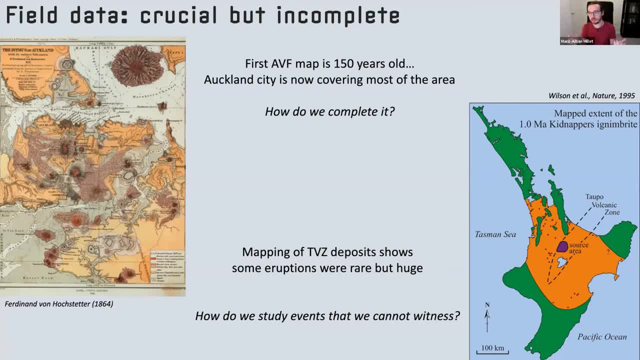 okay, the first, uh, you know, european europeans arrived about, you know, in the 1700s, late 1700s, and that's when the historical records, uh records, start. before that, the maoris that were there, or pacific islanders that were there, actually did not keep historical written, historical records. 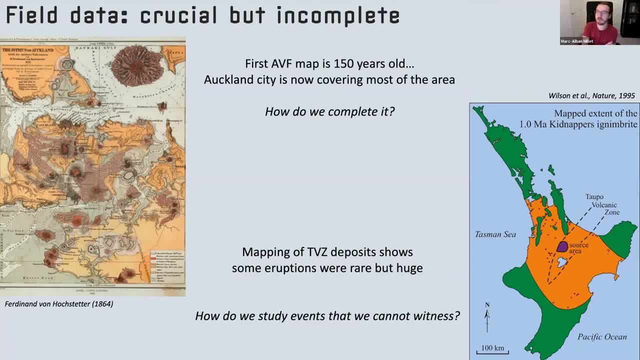 okay, um, and so you know if you look at the top of volcanic zone here. so that's the, the image on the right many of these tvs and top of volcanic zone deposits show. these structures are pretty rare but absolutely huge, and in here i'll just highlight one deposit from one eruption that happened about. 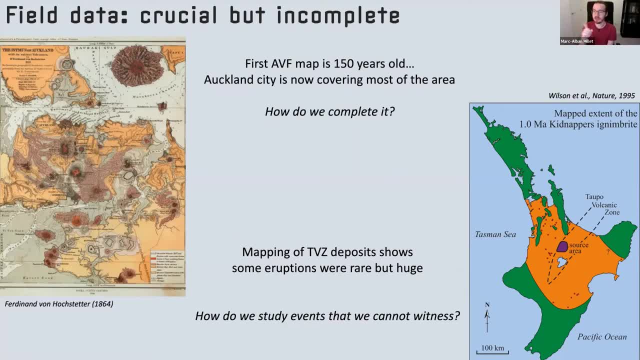 a million years ago, which is called the cape, kidnap this eruption and especially, i'm going to highlight what we call the ignenbright deposit. ignenbright is this volcanic deposit that, rather than ash, that just spewed out and then calmly settles down. okay, this is actually what we call this search, uh, pyroclastic flows that simply 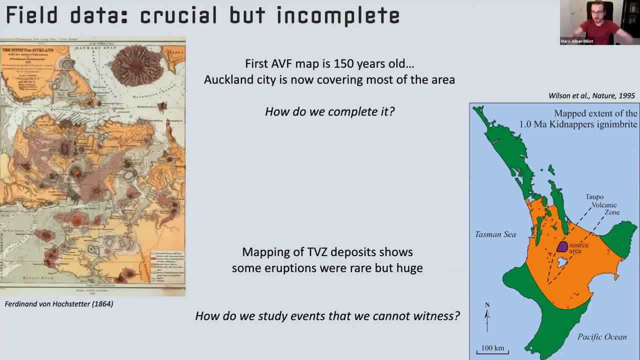 fall down the ash color the, the volcanic column and then just spread on the floor like this. naturally okay, this volcano, this specific eruption, pardon, this specific eruption in- is named after a cave in new zealand that is located here, right there, 300 kilometers away from the vet. and this is because 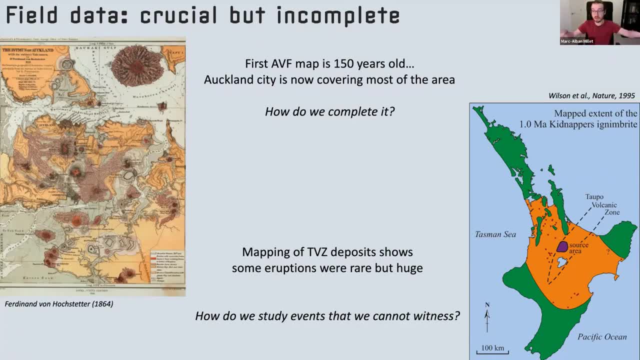 the deposit there of the ignenbreit, this natural surge of, you know, hot, uh, ash and air and ash is actually flowed right up to there across the land and the deposit is still about two meters high. okay, this is absolutely monumental in terms of eruption. okay, so how do we study these events that? 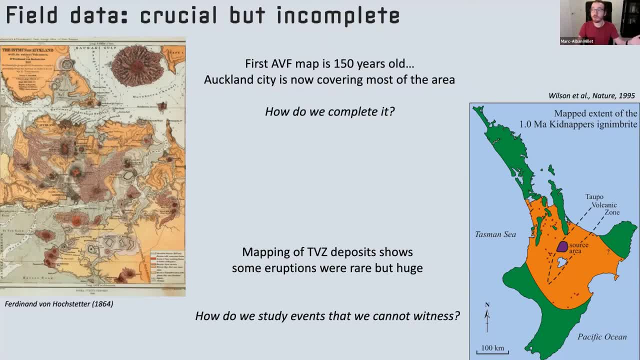 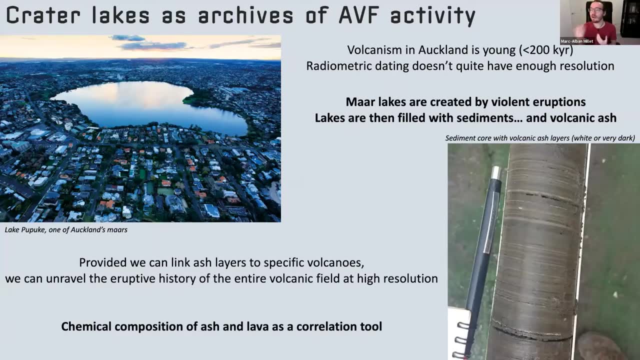 we haven't been able to witness and we have no records of. So I'm going to first focus on the AVF and in here, one way we have tackled this, and I've been fortunate enough in my career to work on both these localities, and this is collaborative work that I've done. 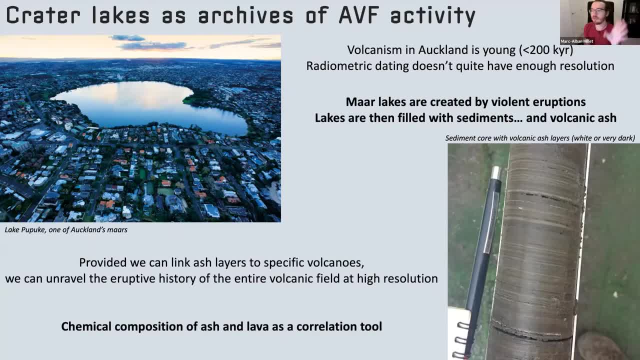 with many people. So in here, one of the things that we have done for the Auckland Volcanic Fields is actually looking at the sediment deposits in what we call the ma craters. So we have these crater lakes in there that have been created by 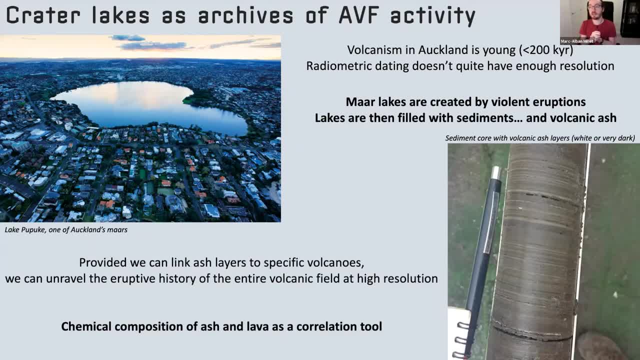 the earliest eruptions, but then, after that, sediments have accumulated in these lakes, and in these sediments we can actually recover the ash of subsequent eruptions. So they've been called, they're taken the boat there, sampled, drilled, tensed. every inch of the suspension, every inch of the sediment. 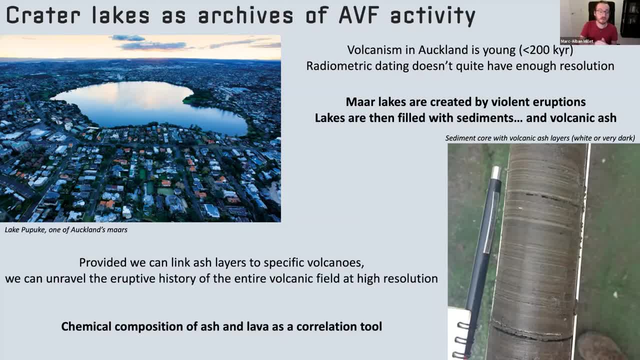 and they're all taken there and the sediment deposits are actually deposited in the ma craters, tens of meters of sediment core to recover this ash And you can see it here. this is a picture of a sediment core that has just been taken out and you can see these white layers there. 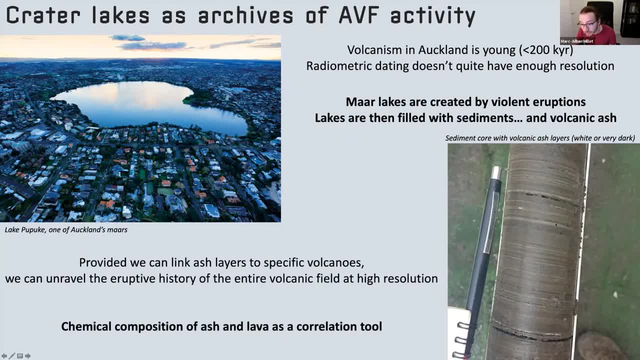 and these slightly darker layers. right there there's one of them. There's another big white layer there and in here. this is actually another coarse dark layer right there. These are volcanic ash layers and they tell us about nearby volcanic eruptions. What we don't know is where the ash is. 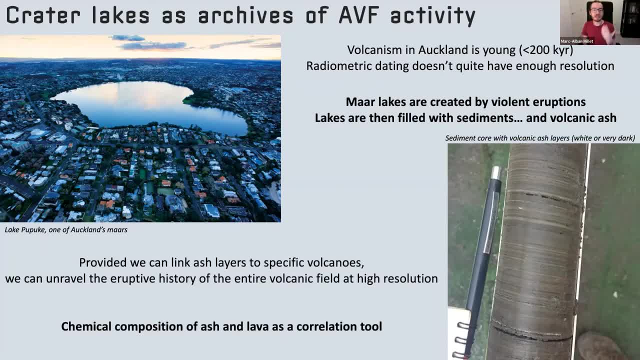 coming from. So you know, provided we can link this ash to specific volcanoes, then actually we can unravel the history of the entire volcanic field. actually quite a high resolution. So in here, what we're going to do, what we have done actually, is using the chemical. 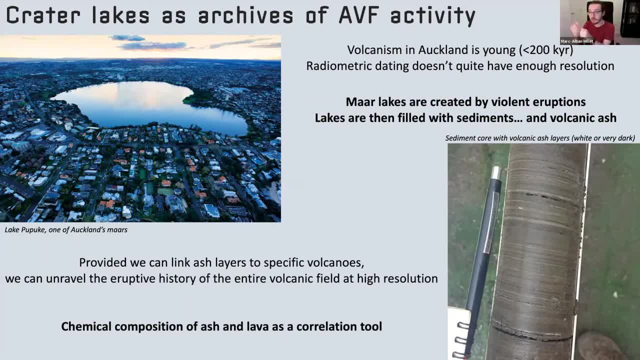 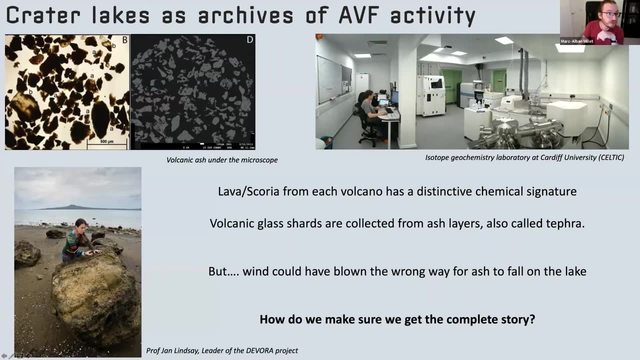 composition of this ash to try and trace it to specific volcanoes that match this composition. So we're going to use this as a correlation tool. And how do we do this? Well, you know, that means that we sample the core in here and we collect all these little glass shards there. 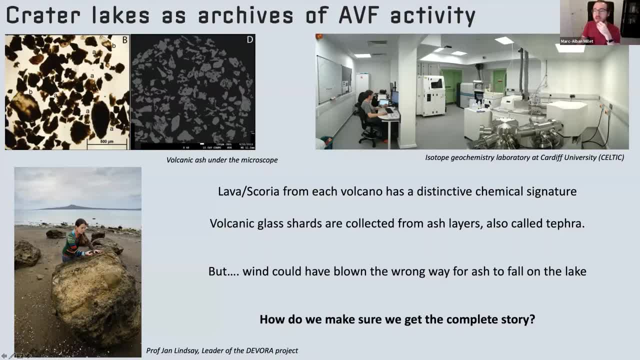 So that's kind of painstaking work there, and then we just bring them into the lab. So this is the lab here. this is not the lab we used at the time. this is the lab that I co-founded in Cardiff University and I'm leading with my- you know- colleague Martin Anderson, who is right there. 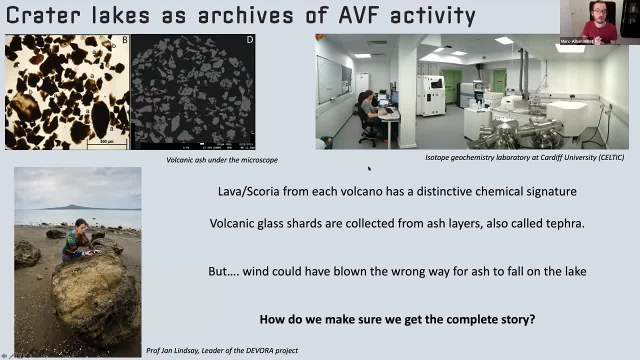 And I would say that you know this, lava and scoria from each of these volcanoes will have, each volcano will have this distinct chemical signature. So, provided we can measure this, this chemical signature, to a high precision, to a precision that is high enough that allow. 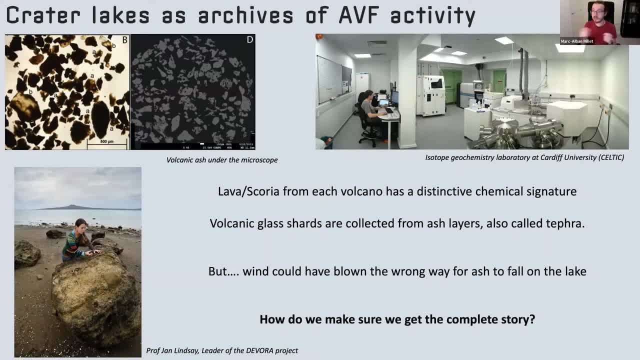 distinctions between volcanoes, then we can actually use them as correlation tools, okay, So, yeah, so what we call those as well is little ash layers. they're called taphras. A downside of this is, of course, you know when the volcano blows. 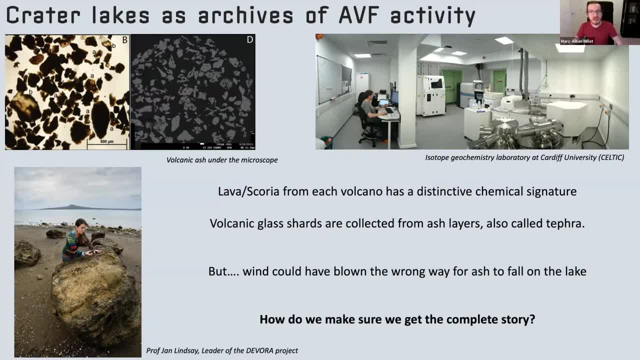 the wind transports the ash, okay, And the wind may have been, like you know, blowing the wrong way and the ash layer doesn't fall into the right crater length that we are sampling, okay. So you know, this is why we need these kind of projects, are actually massively wide-ranging. 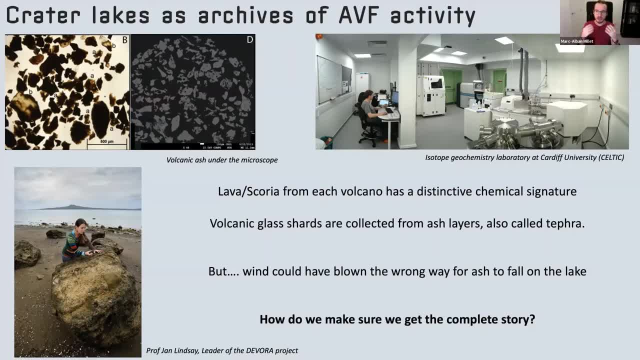 okay, These are, you know, projects that takes a huge amount of people and a large amount of money of public money. So we, you know, we don't want to have a huge amount of people and a large amount of money of public money. So we, you know, we don't want to have a huge amount of people and a 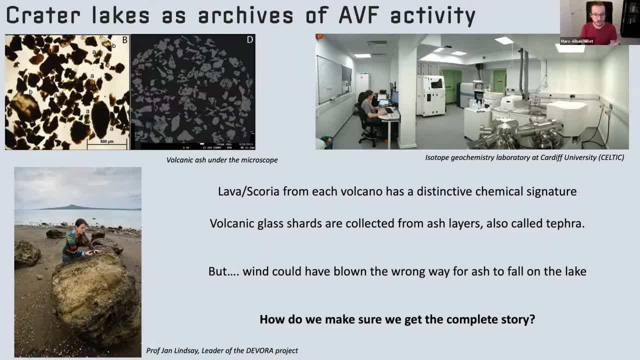 large amount of money, So we need to know that. make sure that you know we're doing things right. And this is a project this year that is led in Auckland. It is led by Professor Jan Lindsay at University of Auckland and it's called the DEVORA project, which is for determining volcanic risk. 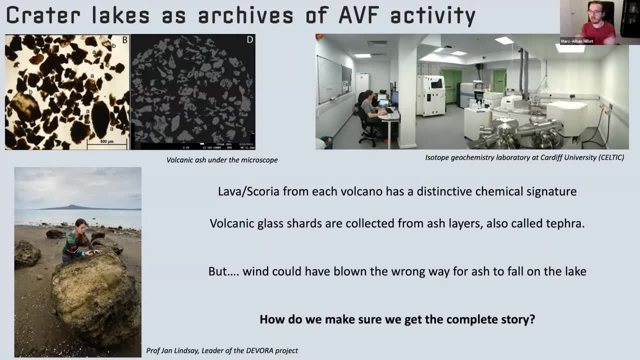 in Auckland, And so you know Jan has done this fantastic job in pulling all this together with elements of social sciences as well- in there- risks, urbanism and this sort of more geology facing approach in there- And she's done a standard job in this. This project is actually 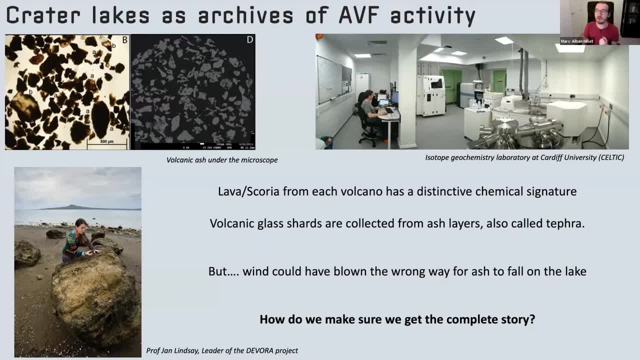 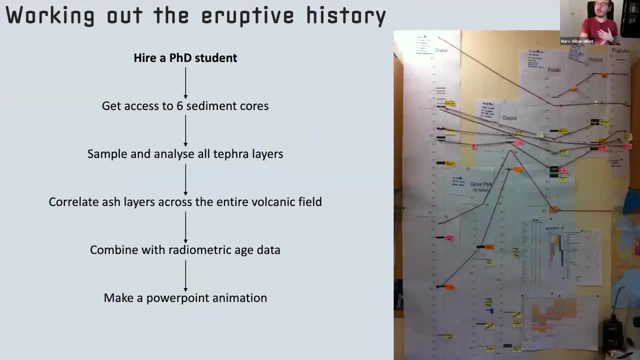 still ongoing to this day. So back to the geology. So you know, we have now collected our ranch. So you know, what we did in this case is that we hired a PhD student to do the job, And then what we did is actually, we got access. 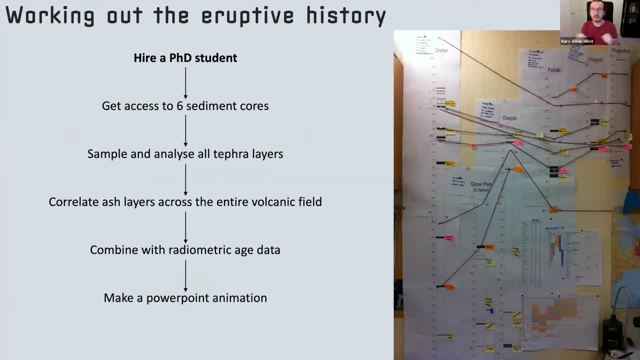 to six of these different sediment cores in different lakes around Auckland- quite circling Auckland in there- And then so she did the sampling. she analysed all the tephra layers and then also analysed the chemical composition of the layers, And then she did the sampling. she. 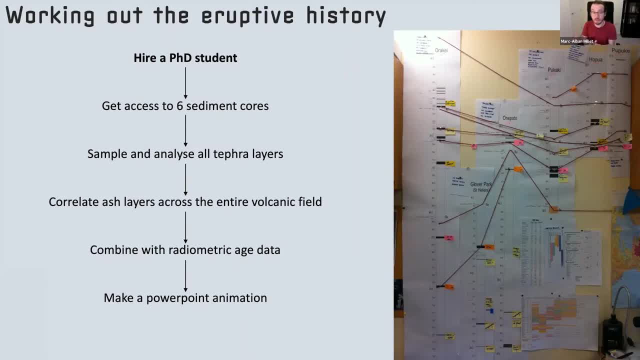 analysed all the tephra layers and then also analysed the chemical composition of the layers. And then she did the sampling. she analysed the chemical composition of each of the volcanoes that we could still sample, And then that was simply correlating the ash layers across the entire. 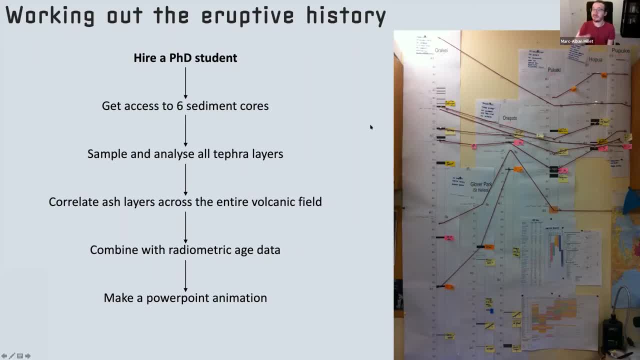 volcanic field And in here this is, you know, kind of painstaking detective work that she did, where these are each of the individual cores with each of the layers that she recorded here in black. these are the ash layers, And then another core here, another core here. 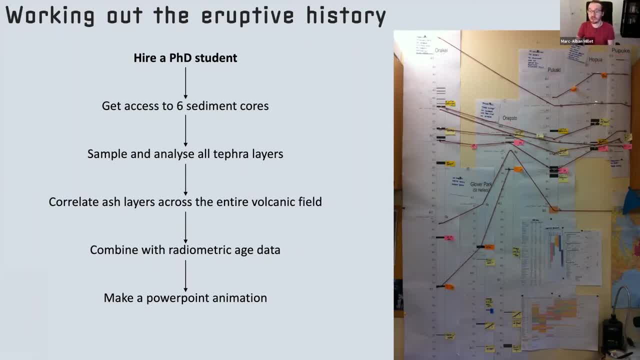 And then she basically said, okay, this correlation, this chemical combination match between: And then she basically said, okay, this correlation, this chemical combination match between: here, this layer, and this layer here and this layer here. this is the same. 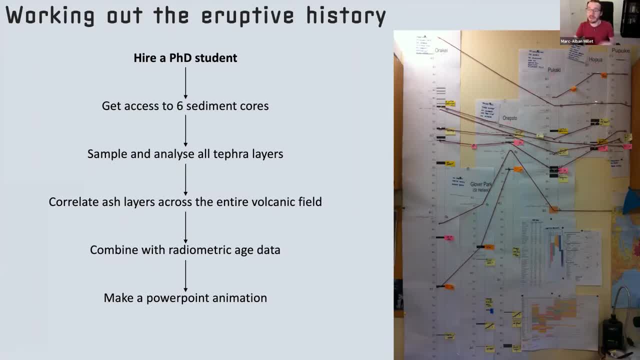 ash layer that can be correlated across different cores, And this allows us actually to sort of relatively time these sediment cores and get an idea of the ordering of these volcanic eruptions at the very east. Okay, What we also have done is that, you know, we can get an idea of the 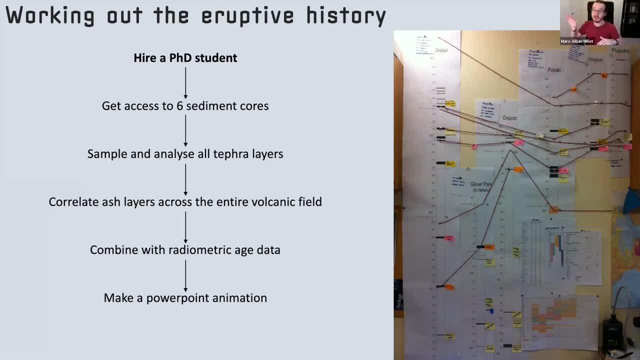 relative dating of these eruptions that way and which volcano they come from. And then we go to the volcano and we date it using radiometric technique, such as Arvan Arvan, for example, And at the end of the day, so this is, like you know, three, four years of work for her. 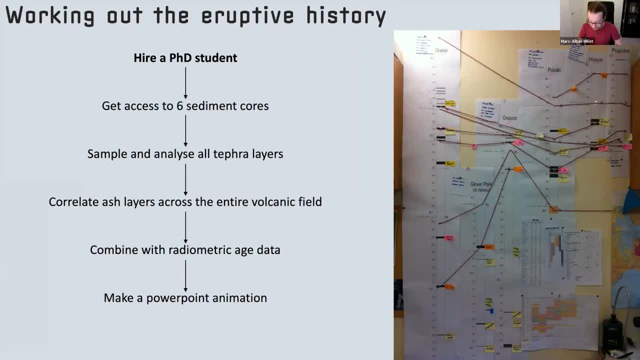 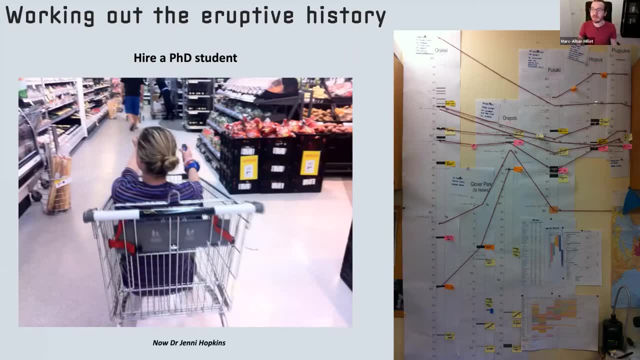 just to do that, And at the end, well, she'll put it nicely in a PowerPoint animation, which is there. I will point out that this is Jenny Hopkins that has done this work under my supervision. okay, Jenny doesn't like to be taken in picture, and so that's the best. 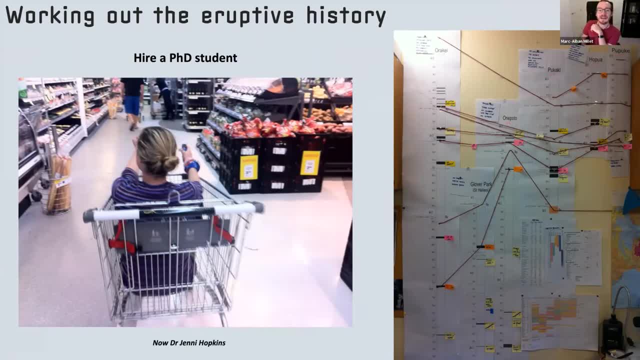 picture I could get of her still to this day And so, yeah, she has done this animation here I'm going to present to you. It's going to last about 30 seconds to a minute, but that shows you essentially what we could work out of of how volcanic activity evolved in Auckland over the 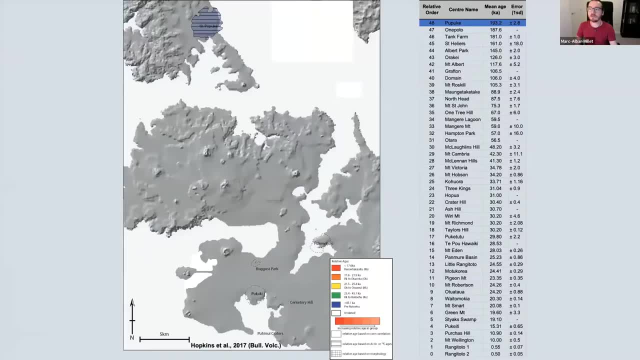 last 200,000 years. There we go, actually going now there. So it started up in the north there with this volcano called Pupuluki and Onipoto, and now we are down to about 160 million years. 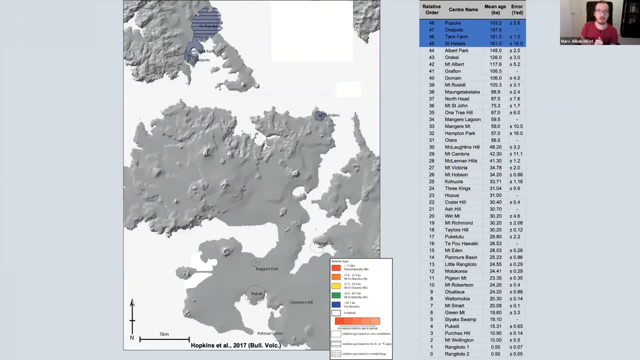 and then it moves now to basically the central part in there- Albert Park here. So it started up in the north and then moved gradually south, originally in the Turisha Centre. Each of the these are the volcanoes there that we are highlighting. 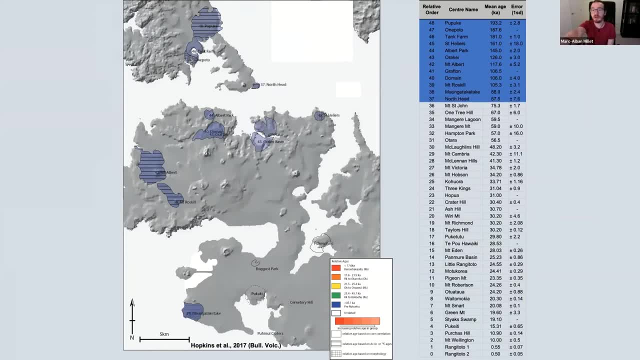 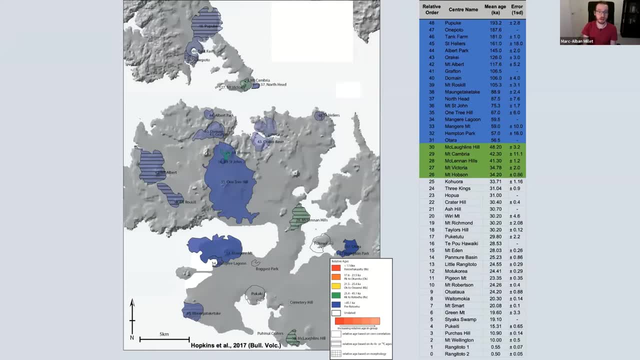 So you can see, now that there's more and more volcanoes, it starts to accelerate. actually, Over the last 60,000 years okay, and we know we're still only about halfway with 30,000 years to go- and now really between 30 and about 20,000 years ago really, we had a burst of volcanic. 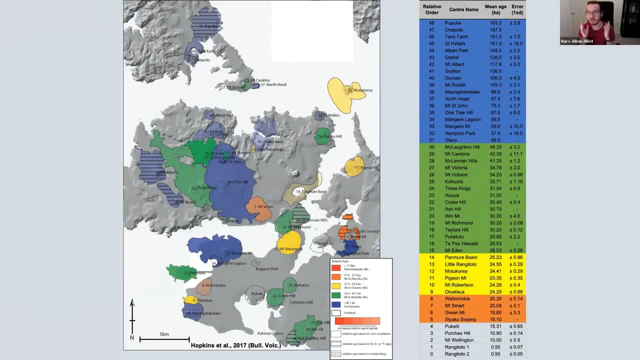 activity, with quite a lot of volcanoes around Auckland being generated, okay, being erupted, Okay, And now it seems to have died down a bit. so there hasn't been only one eruption over the last 10,000 years. However, this is also the biggest one. So is it because the field is? 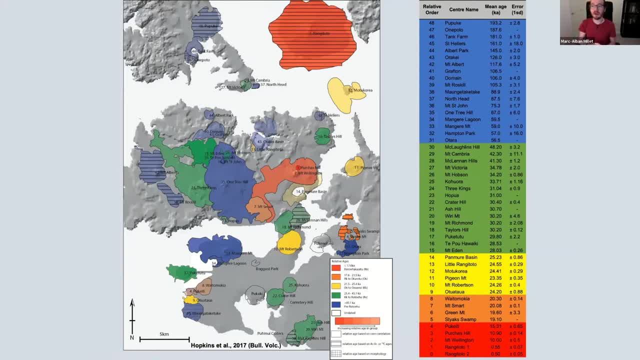 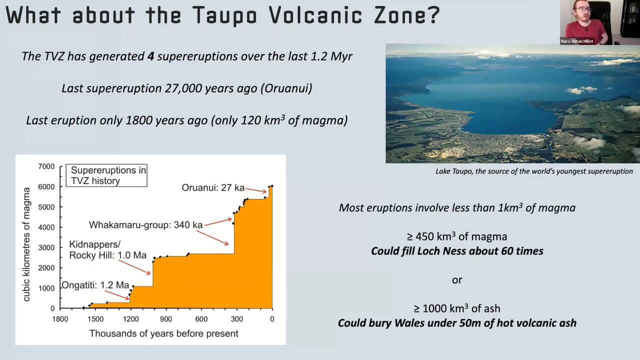 changing in terms of its behaviour? or was it a last hurrah? We don't know, and that's why further research is actually very much needed in this project. This Devora project, is still very much ongoing. One thing now, like I'm going to switch to the second part, is: you know what about the 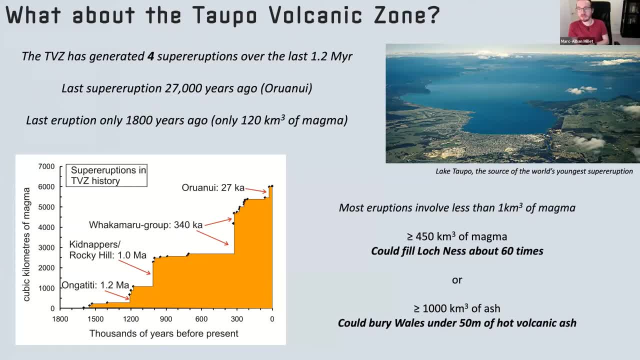 Toa Apu volcanic zone. So that's a completely different volcanic system in New Zealand that is completely much less frequent but with an eruptive behaviour that is so much more destructive. Auckland's very small volcanoes, in the grand scheme of things most of them quite effusive. 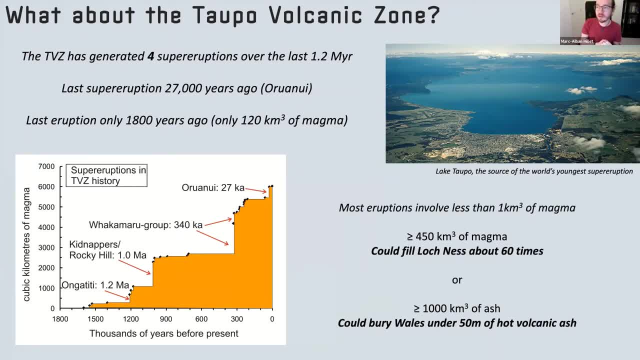 the lava is, you know, quite running down. There are some slightly eruptive, explosive ones, but not very much, not to the scale of the Toa Apu volcanic zone, which has devastating eruptions. Okay, So this Toa Apu volcanic zone has generated, amongst others. there are other eruptions in there. 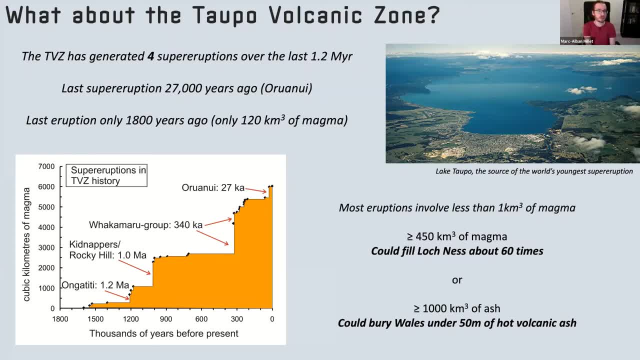 but four super eruptions over the last 1.2 billion years. okay, with the last one about 27,000 years, which is called Oruanui. Okay, The last eruption, which is not a super eruption but a significant eruption, still was about 1800 years ago And, to give you an idea, 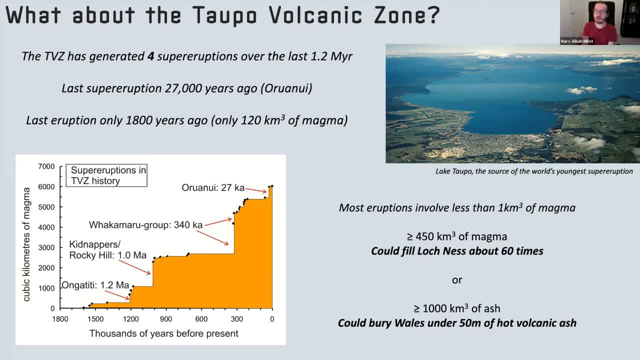 what we call a super eruption is about 400, over 452 kilometres of magma. okay, 450 kilometres of magma could fill the Loch Ness about 60 times over, right? So we are talking about an eruption that instantly or within weeks erupts a volume of magma that could fill the Loch Ness about 60 times. 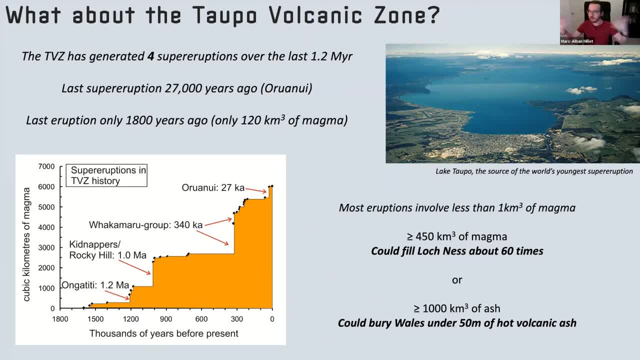 Or if you want to put it as an ash layer, so to note, that's the eruptive product at the end. so we should compare the volume of ash. that's about a thousand kilometres cube of ash. So if you want to do it from a Welsh perspective, this could bury whales in about 50 metres of ash. 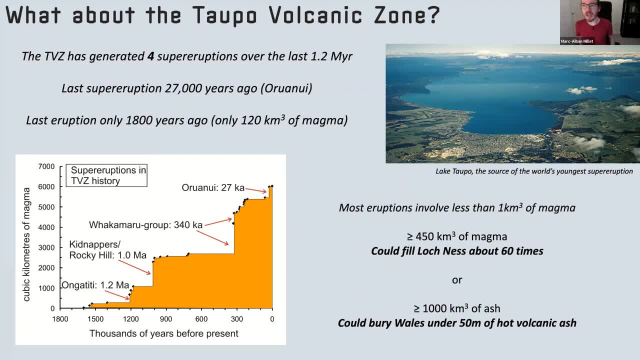 of hot volcanic ash instantly. We are talking here about absolutely massive volcanic deposits. okay, The last eruption was about only 800, 800 years ago, but you know only 120 cubic kilometres of magma, so not a super eruption, but still devastating enough. I've seen the deposits of 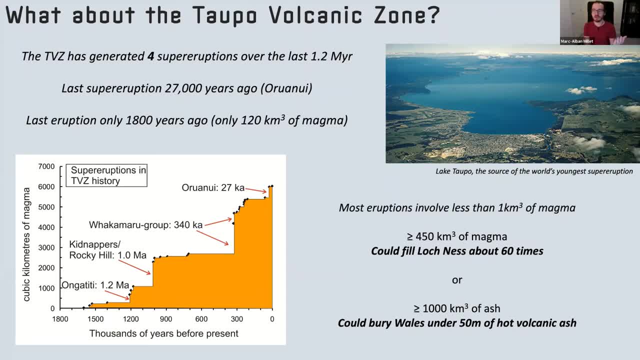 these eruptions. I've shown students this, these deposits, for years and you know you can find them hundreds of kilometres away and they are still very sizeable: deposits of several tens of centimetres to several metres, something that would you know to nowadays would be absolutely. 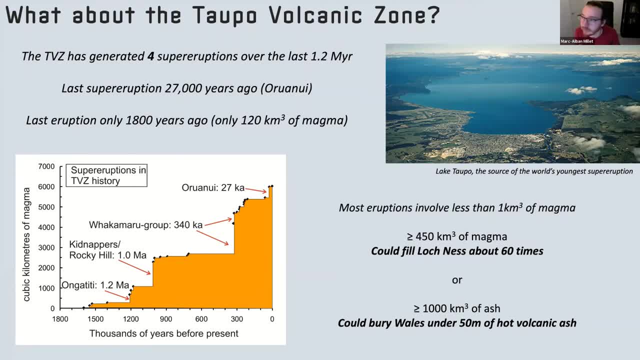 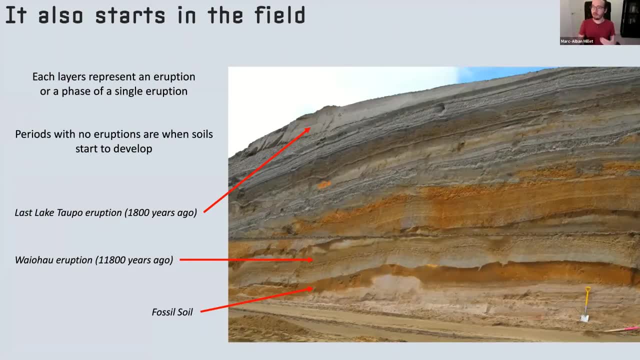 devastating for human life And for any economy, for that matter. okay, So how do we tackle these? you know slightly different deposits. Well, again now we're going to go this time to. you know, look at the field data. it starts always in the field. in this case, 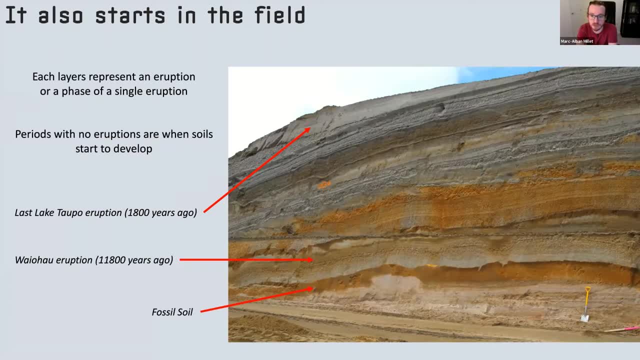 Each layers in here. so these are multiple layers of ash, of volcanic ash. each layers represent an eruption or the phase of an eruption, because not all eruptions are going to be necessary. but they are going to be necessary because not all eruptions are going to be necessary. 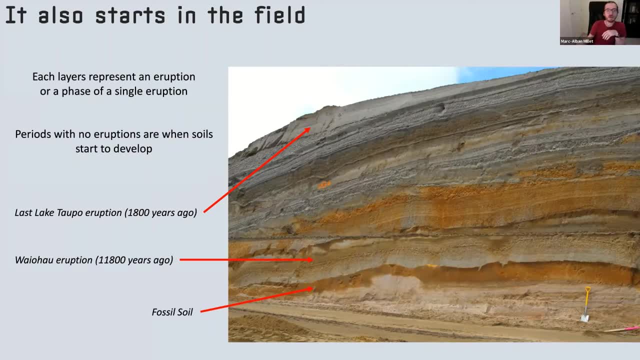 continuous okay Periods with no eruptions are not simply not recorded, they are on purpose, when the soil is actually might start developing okay. So in here, the top, at the top of this outcrop, here you have this layer here which is the 1800 years ago temple, like the last lake temple. 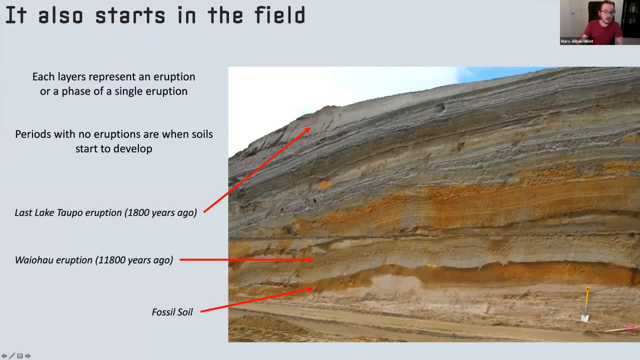 eruption which is called the Hatsipi eruption, And in here you have another one here which is about 1200,000 years. this is this eruption there, And you know when I was talking about- sorry, when I was talking about, you know. 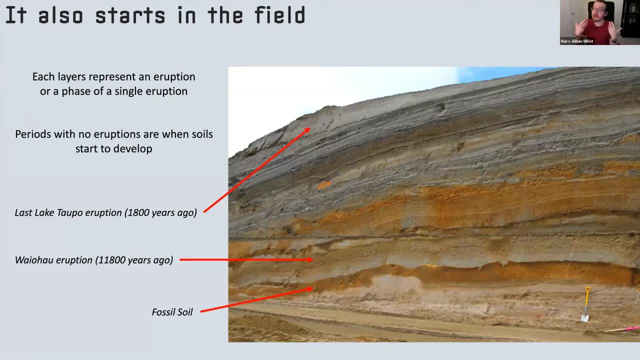 what happens when eruptions actually do not happen, but instead they have soil developing, And this is what we mean by soil developing. this is this orangey colour. in there, the ash, which is mostly silicic, high silicic, so white- actually starts this colour, and you know. 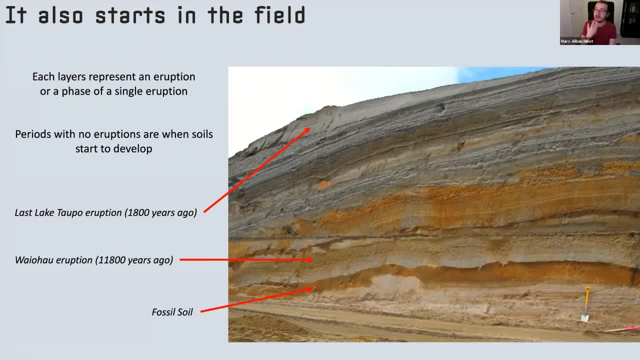 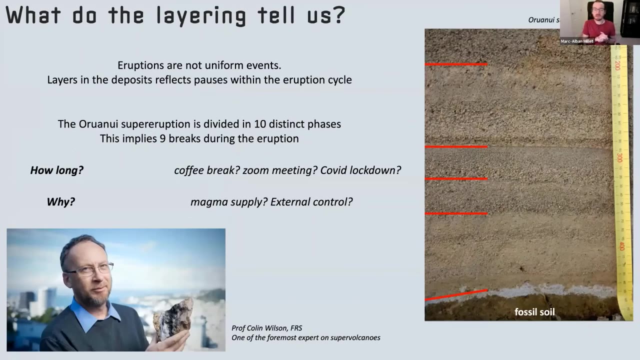 the iron starts to get lished out. the iron gets left behind. that gives this orangey colour. So that is a paleo soil, soil, essentially, that is developing. So how do we read that code? again, I want to say that, you know, to this work was mainly done in. 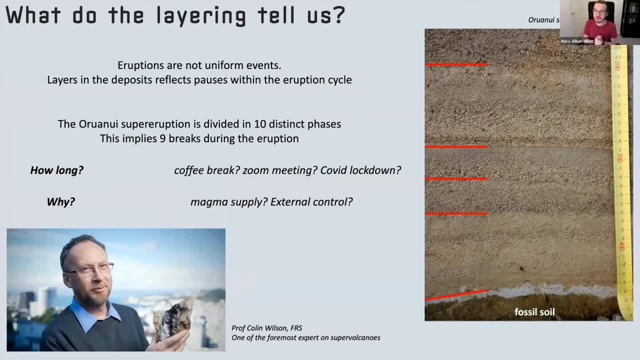 collaboration with Professor Colin Wilson, who is a fellow of the Royal Society and he's one of the most foremost experts on supervolcanoes and he works in Wellington there And I did this work with him and a PhD student again that we were supervising together. on the youngest: 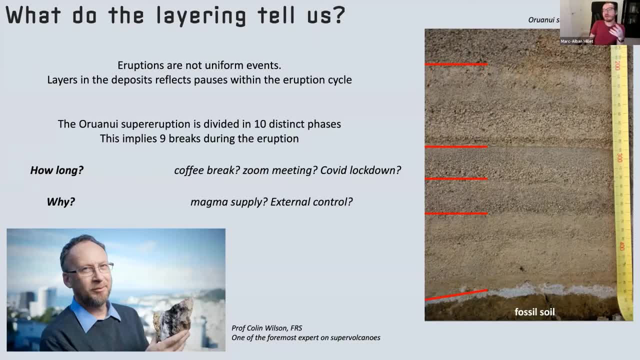 supereruption on Earth. So these kind of supereruptions they're not uniform events. they are so massive they have their own structure and their own history. okay, But the layers in the deposit reflects what we think are poses in the eruption. 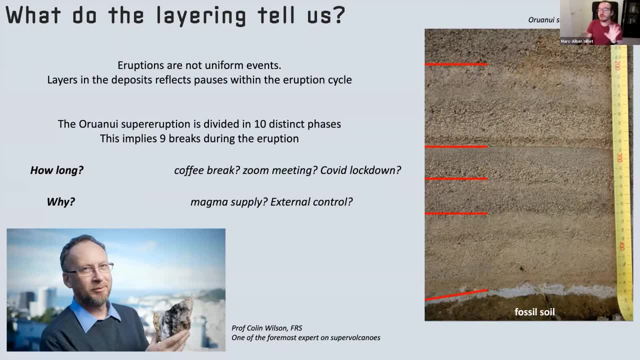 cycle. okay, And in this Oranuri supereruption deposit, you know the 25,000 years old one. what we thought is that we identified these 10 distinct phases in the eruption. That means that if we have 10 distinct phases, we also had nine breaks. 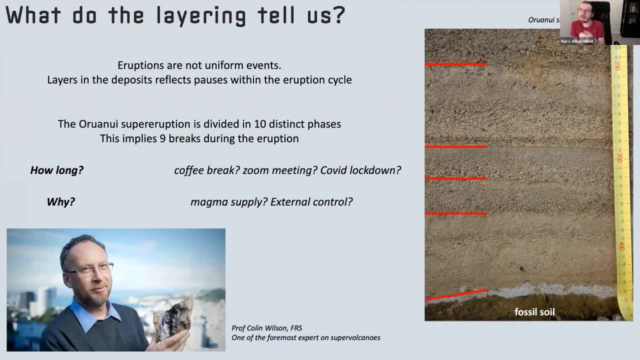 So what are those breaks? How long are they? Is it the time for you to make a coffee, or is it a lockdown, for example? that has been going on for weeks and months, And why is that actually? Why do we have these sort of pauses and starts and stops? 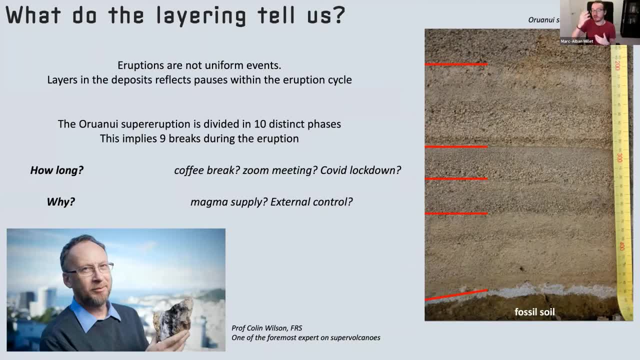 Is it because the magma supply actually in the magma chamber is waning and coming and going essentially, Or are they external control on the magma chamber whether it can actually vent or not? You know, is it the crust inside that has stresses on it? 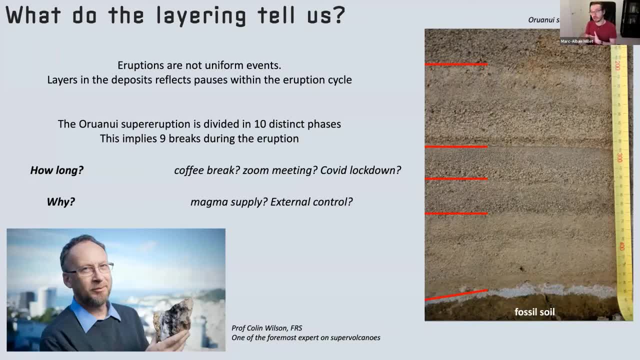 that you know, that is stopping or promoting eruptions or stopping them. And in particular, in the next few slides I'm just going to talk about in here this very first small layer. okay, This is a fossil soil here. So we know that's. you know before that that's the 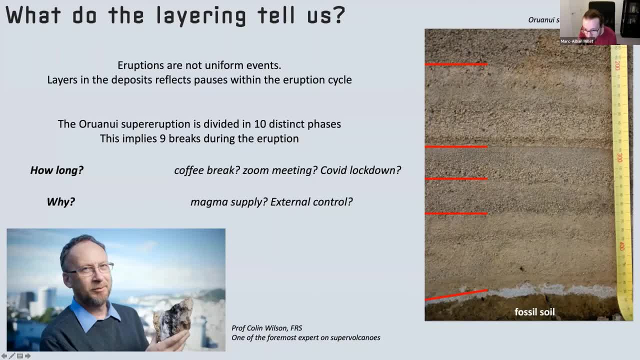 eruption is at the bottom of this layer, right there, if you follow the mouse there, And then we have this bright grey layer here and there. that is actually, you know, a bit discontinuous And that's the reason why we think that, if there is not, this deposit has been reworks. 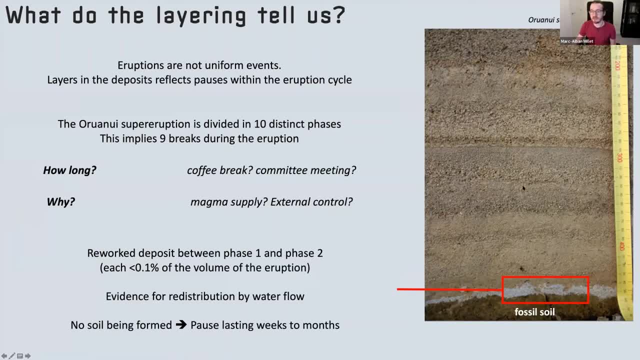 And that's what we call the phase one of this eruption and the rest of it is actually phase two. Okay, So what we see that have been mapped after that, this phase one of this deposit, Colin has done this extensive work in mapping these, in finding these starts and these phases and mapping them. 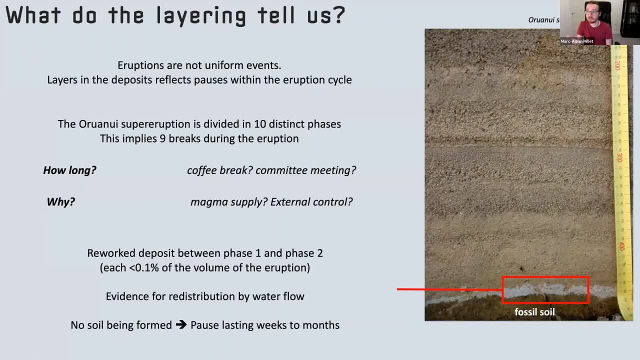 is about less than 0.1% of the volume of the eruption overall. So it's really really tiny that phase one. But what it did, it's been reworked, So we have this evidence of redistribution, but no soil has been formed. This layer is actually still bright grey. 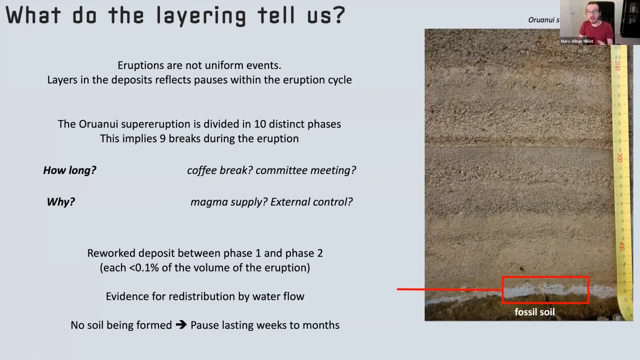 That indicates to us that this pool has been long enough for water to be able to flow on it, but not long enough for the soil to develop, And that indicates weeks to months, not much more than that, otherwise you would have the soil starting to develop on it. 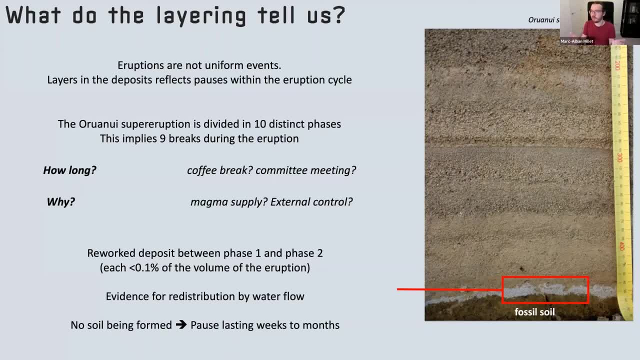 not much shorter, otherwise you wouldn't have had the time to actually rework that deposit. So that's the evidence. So that's the evidence. So that's the evidence. At the weeks to months break, How do you do that? You have a. 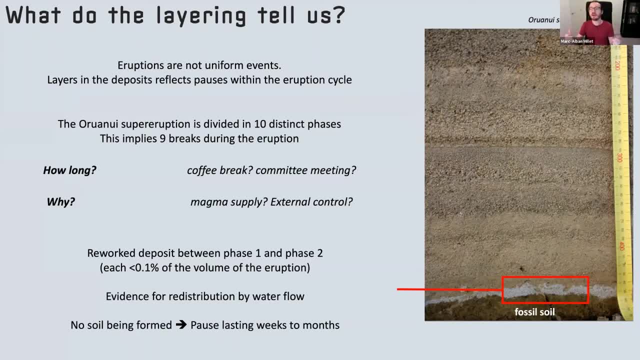 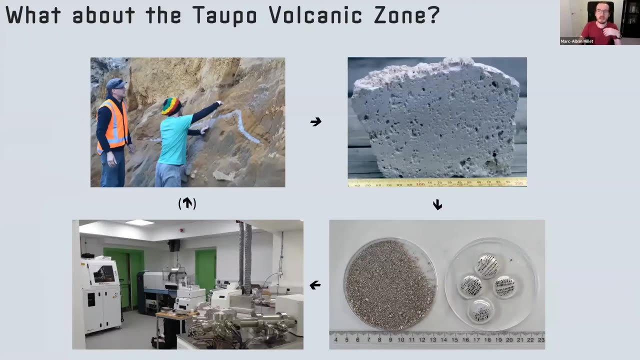 pocket of magma, a huge pocket of magma that is ready to blow, And you just let out a tiny amount and stop and stop the tap. switch the tap off straight away. How does that happen? Well, again, so we take students here. This is Alastan, and I was too talk in these deposits. 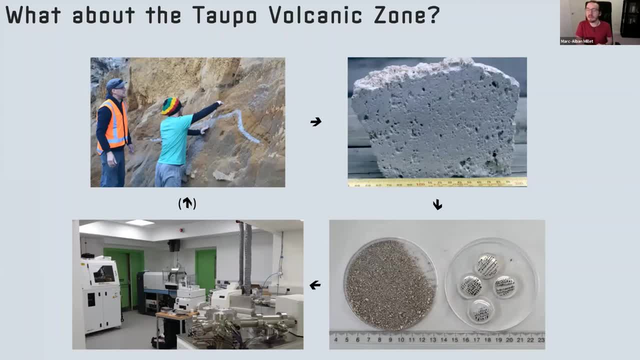 And what he did is actually collected a lot of the premises Okay, And in the permits. What he focused on is many crystals in their phases and especially pyroxenes, because their chemical composition takes a lot of trace elements, chemical elements in them and they can be really useful to actually trace down the chemistry of the magma and its evolution. 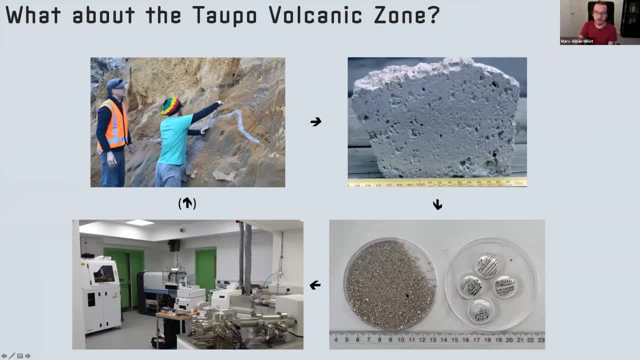 So what he did is that he took these pumice from the field, crushed them and then picked out all these pyroxene crystals and then laid them in epoxy mounds to be taken into the lab and analysed. This was really painstaking work. and then do that on repeat, of course, because we get some work done. we get the field, get some samples, get some work done on them, learn from them, then target another area, another locality for further work. 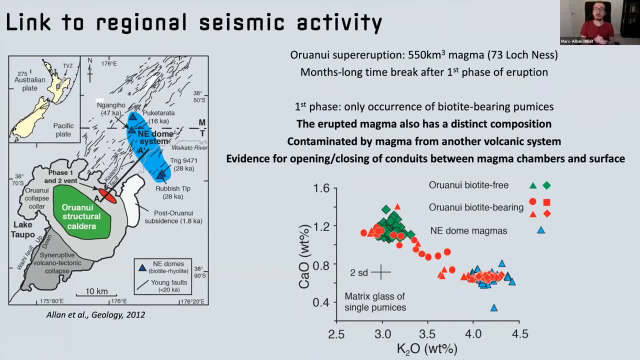 And what did he learn? Well, okay, So we're looking at the Euronewes supereruption: 550 cubic kilometres of magma, massive 73 Loch Nessus, And we have this months long time break between after the first phase of eruption. 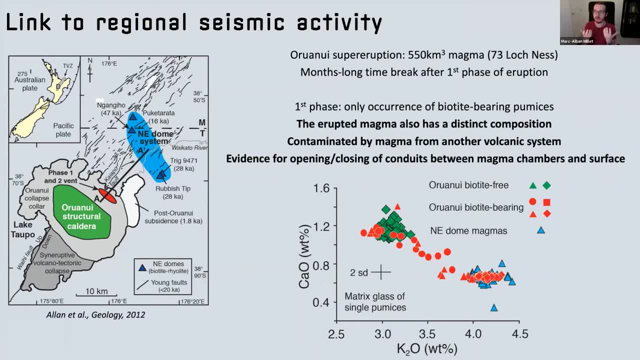 What he did find, though, and one of the questions that he was trying to answer was: how does that happen? is that this first phase is also the only phase in this whole eruption where we have a specific mineral called biotite. This is the only time that we have biotite. 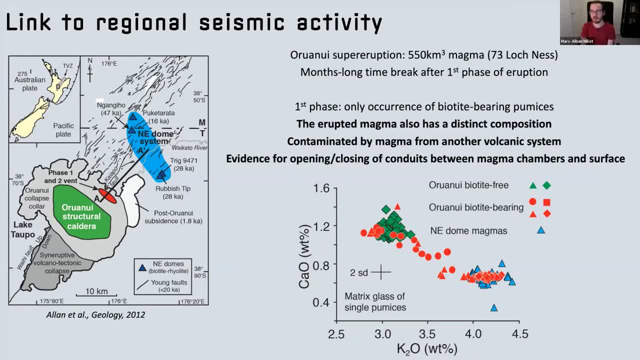 Okay, And we have biotite included in that specific volcanic deposit, So that makes that first phase even more unusual in the context of this supereruption. Okay, And so this map has this distinct composition, And what we did find is actually that we analysed the deposits from another volcanic system, which is called the North East Dome System, which is about 15 kilometres away from the Lake Tarpon. 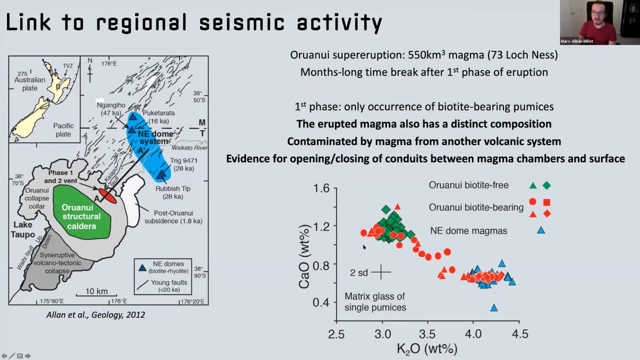 And it actually matched. Okay, And what we did see is that- and this is in the plot of the calcium content versus the potassium content of the glass, actually of this pumice, is that this is all the pumices from phase two to phase 10 of the Euronewes supereruption. 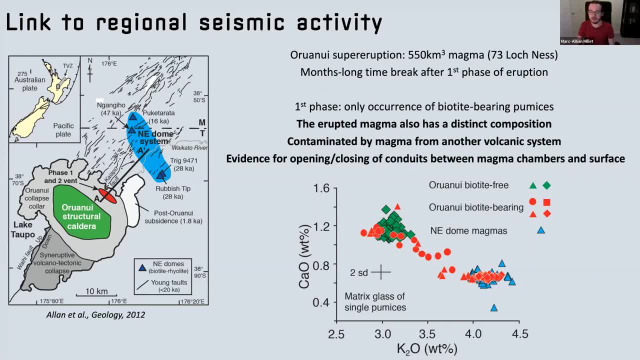 We can see that they all clustered together They are very invariant. This is in blue here, the blue triangles. all the pumices from the North East Dome System. Okay, But if you look at the phase one pumices, at the glass in the pumices, they are very invariant. 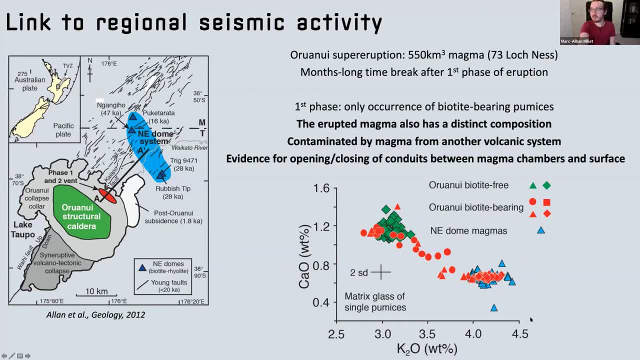 Okay, But if you look at the phase one pumices, they actually range in between the two. So what that means is that that phase one, the magma erupted in, a phase one of this eruption was actually contaminated, a mixture between magmas that were from the North East Dome System and magmas from the overall Euronewes structural calera system magma chamber. 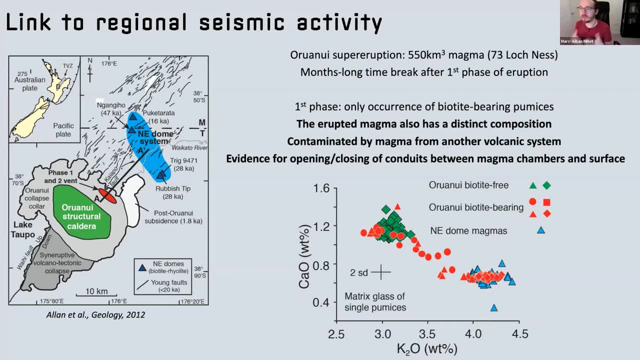 Okay, So we do have evidence of contamination and essentially a plumbing system that was active in between these two magma chambers. Okay, So, we do have evidence of contamination and essentially a plumbing system that was active in between these two magma chambers. Okay, So, we do have evidence of contamination and essentially a plumbing system that was active in between these two magma chambers. 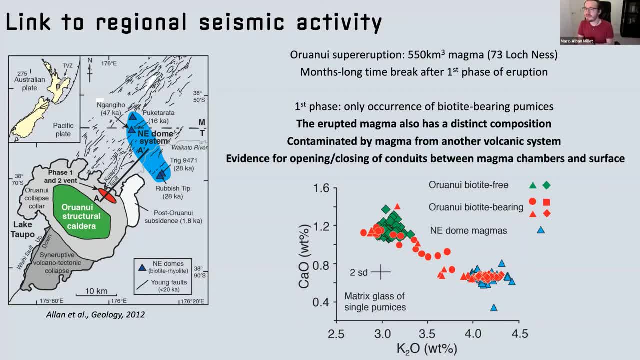 When people check and we found that these two magma chambers of the plumbing system to an extent that magma could actually mix together and then erupt, And then those septic structures must have relapsed somehow after this crisis of seismicity and they closed again. 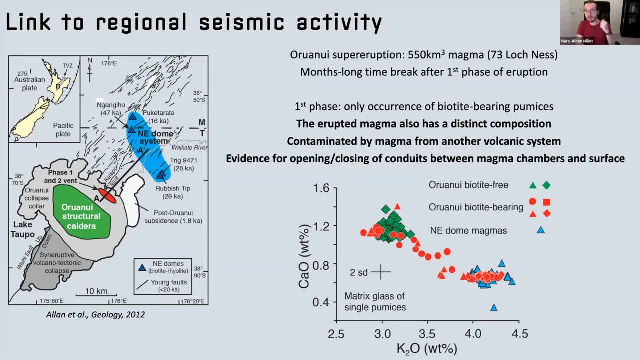 But by then the magma was probably really primed to erupt, and then, when it blew up a few months later, then it went for good. This is what we think happened. So this is my last slide, and I hope I've shown you or piqued your interest. 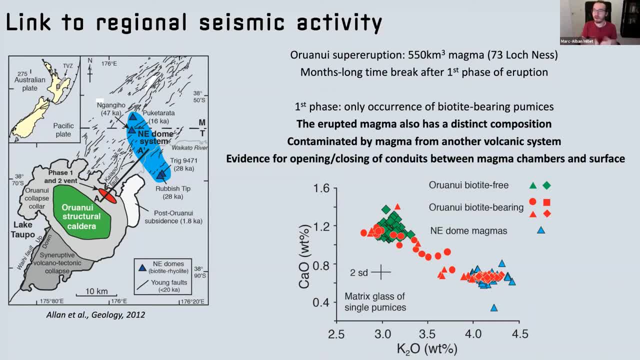 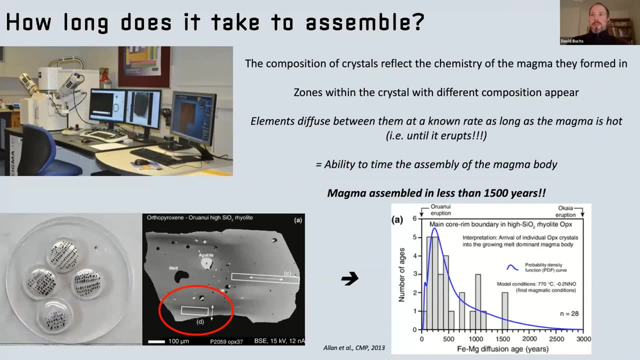 in how geologists can actually understand big volcanic eruptions or volcanic eruptions in a wider context. And yes, I'll very much happily answer to any of the questions that you have. Thank you very much. Thanks a lot, Marc-Arbonne, for that very interesting talk. 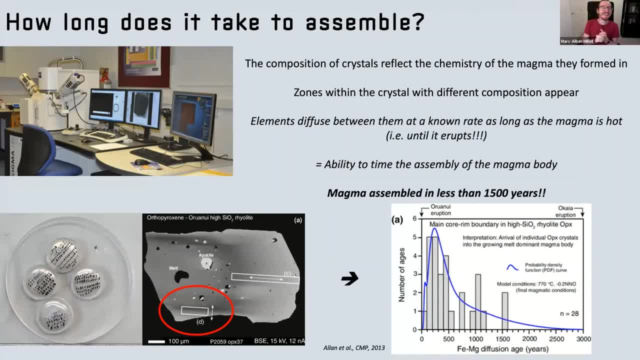 Oh sorry, I just had one more slide. So basically the question was actually: you're talking about super eruptions, but how long does it take to assemble one? Do you take millions of years, tens of millions of years, or is it actually much shorter than this? And when we talk about 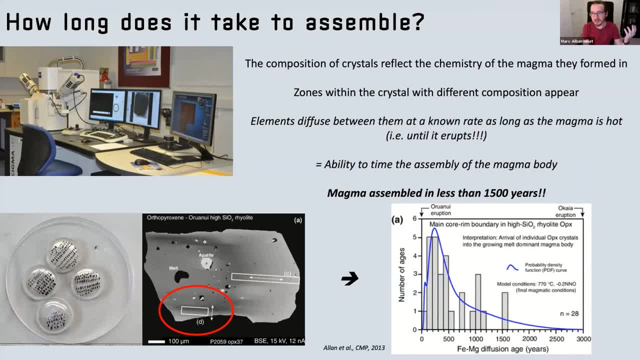 volcanic eruptions that humans have never witnessed, then this is becoming an extremely important question. So this is also part of Aidan's work there. So what he did is actually took those little pyroxenes that I mentioned earlier a few slides ago, and he imaged them in this way we call an electron. 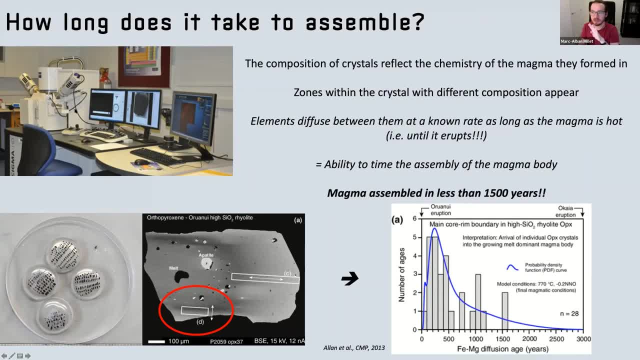 micro-probe. An electron micro-probe is very good because it can give you this contrasted black and white image that are sensitive actually to the chemistry of the mineral in question. And in here it's actually the ratio between iron and magnesium here that we are imaging with the 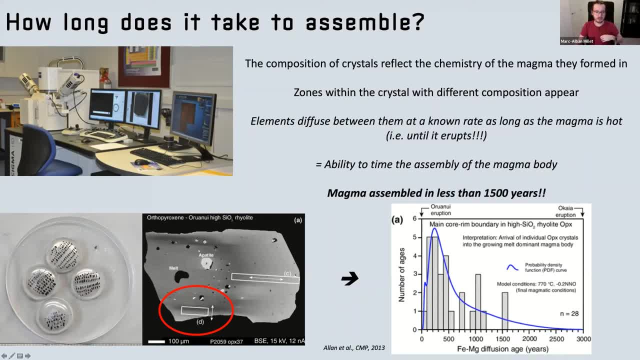 contrast, with the lighter colour being the more iron rich, yes, and the darker colour being the more magnesium rich. So what we see here is that what we call. we have a zone crystal, and the zone crystal actually just tells you that the magma composition has evolved throughout. the crystal has been formed. 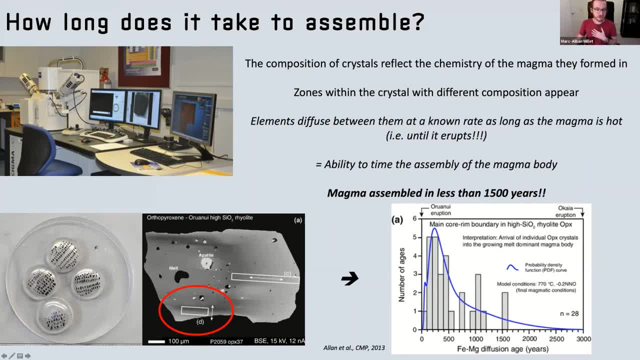 in the magma that had the change in composition through time. Okay, this core of the crystal is the older part, the rim here is the younger part. So it grows. it grows, but it grew in the magma that had a change in composition. What is really key here is that iron and magnesium actually try. 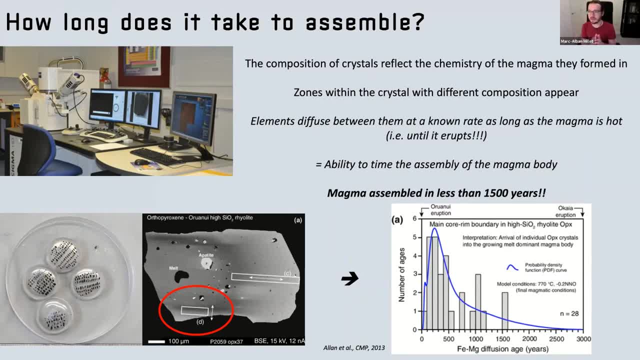 to re-equilibrate. they don't like to have to be in a crystal that has this viable composition. they like to be all the same, they like to be evenly distributed, And so they do this re-equilibration by a process called diffusion. And diffusion is great because it is time. 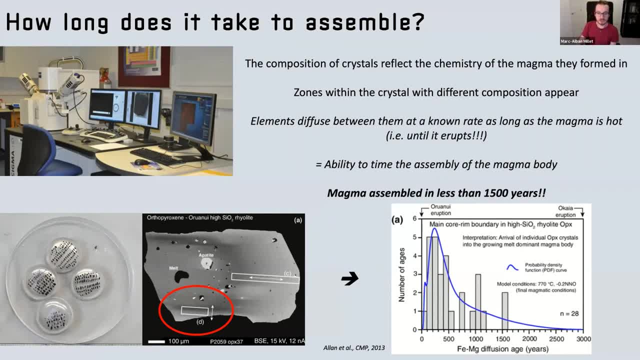 sensitive. we have a clock there, And what we can do here is simply take an idea of how diffused these boundaries are in here And now. we can then actually have an idea of how diffuse these boundaries are in here And now. we can then actually have an idea of how. 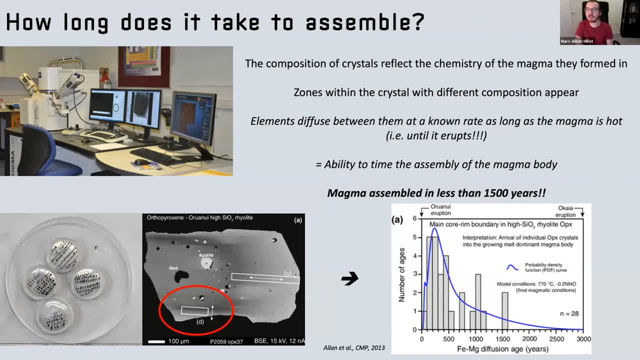 diffused. these boundaries are in here And now. we can then actually have an idea of the time, of the residence time of this specific crystal in the magma chamber. Okay, this is. this is really really good information for us. So, of course, like you know, there's a lot of you know. 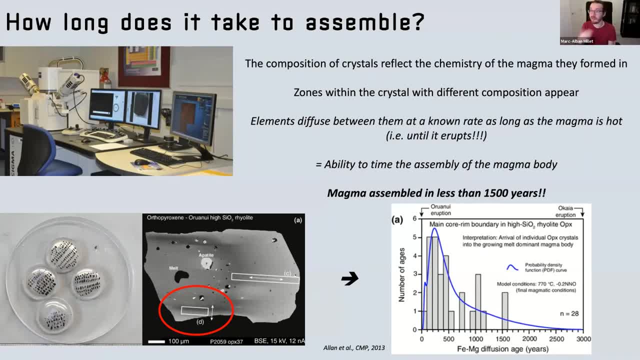 uncertainties in there. So what you need to do is actually take a lot of pyroxenes and then you know, see, see how much if they give you a consistent denser. And so this is why he picked so many pyroxenes for a single sample, And so in basically what he did here, so he did all these. 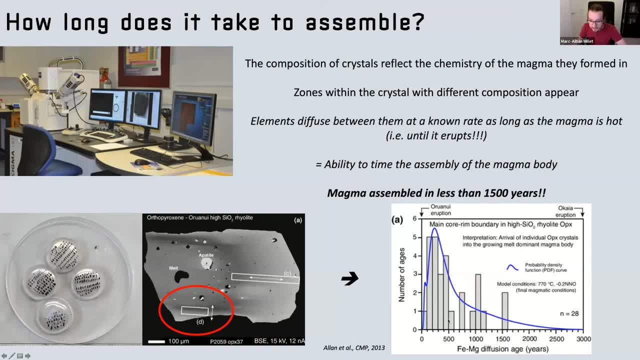 what we call diffusion ages, And this is a probability plot. So this is all the results given in there, And what we see is that now you have a lot of these ages that are around 300 to 500 years, but some are coming up to about 15, 1500 years. This is the oldest age he got for that. 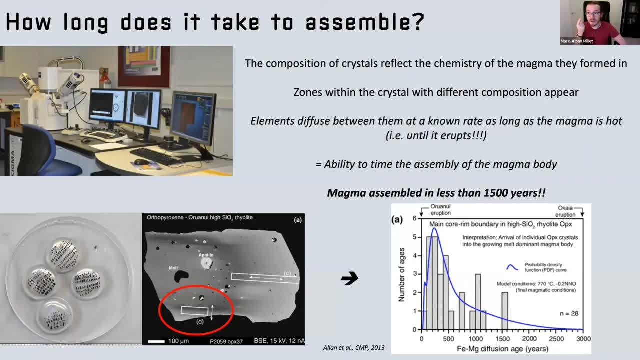 super eruption. What he tells us is that the eruptible magma body that you know, the magmas that ended up being erupted, the magmas that ended up being erupted, the magmas that ended up being- was formed within less than 1500 years, And we are talking about one of the most significant 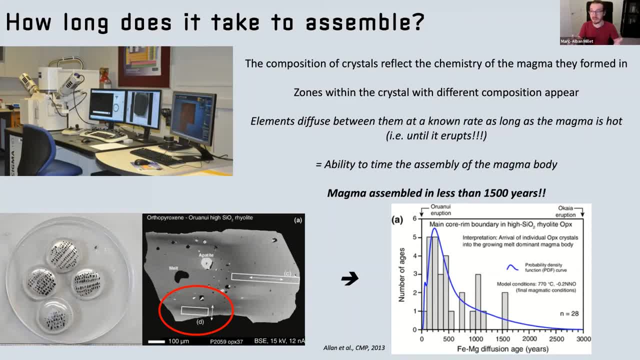 eruptions of the last 100,000 years on earth, something that would devastate an entire country. So these, these big super eruptions, absolutely you know we don't see them on human timescales, but they are actually building on human timescales So they can be actually very, very dangerous And 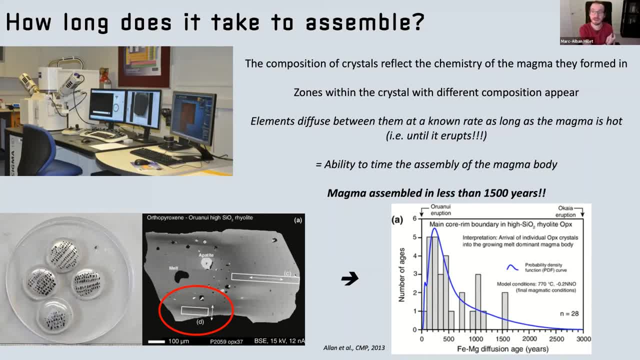 you know, we could have one building up right now that we don't quite know about, Okay, So, yeah, so I think that's it now. I'm nearly done. I am done And, yeah, I'm looking forward to your questions. 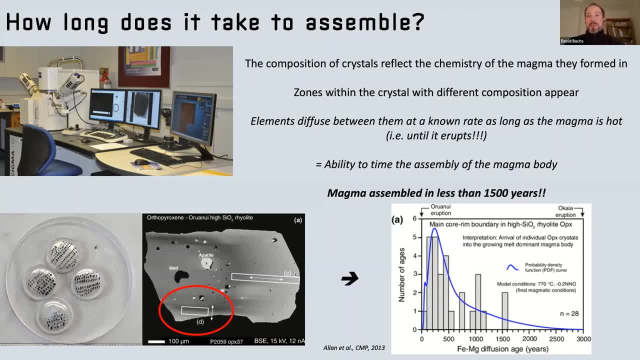 All right, great. Thank you, Marc-Albon. So yeah, that was a nice compliment actually to your earlier talk. So I think there are some questions coming through which I'm going to read for you. The first question is about diffusion in crystals. So is diffusion in the crystal affected by? 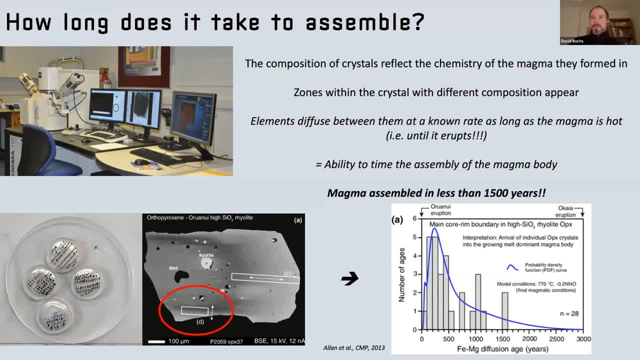 temperature and pressure. Yes, it is affected by temperature, So we need to have an independent constraint of the temperature of the magma. That is absolutely correct in here. So you know, what we do is actually use crystals that are actually in equilibrium with the pyroxenes that we know formed with from the same 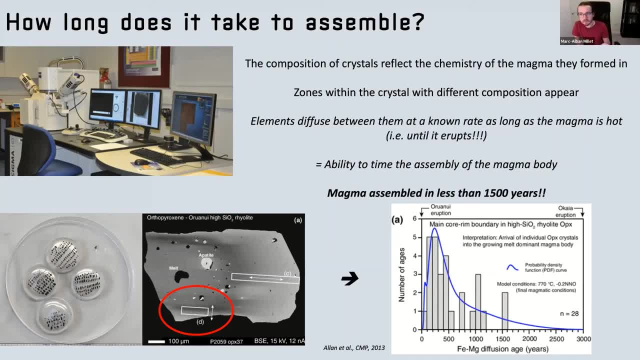 magma to get an idea of the temperature. And this is why what we do here is this diffusion actually stops really, usually under 700 degrees, 800 degrees, its diffusion becomes extremely slow and essentially stops. So this is why we are timing the formation of this crystal, but we are timing the time between the formation of 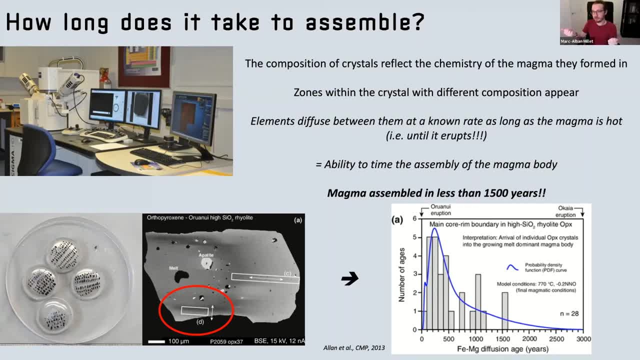 this crystal and the eruption, and not between the formation of these crystals and the present time. It's because once the magma is erupted, it cools down and then the diffusion clock stops. Okay, Pressure? no, It doesn't. pressure does not affect all diffusion, or to a very secondary. 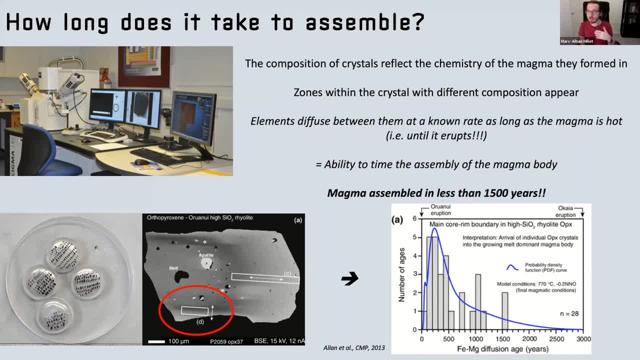 extent. So the range of pressure variation that we have in magma chambers would be insignificant effects on the diffusion timing. Great, thank you. Any other question? So please feel free to use the Q&A option if you want to ask other questions. I've got a question. 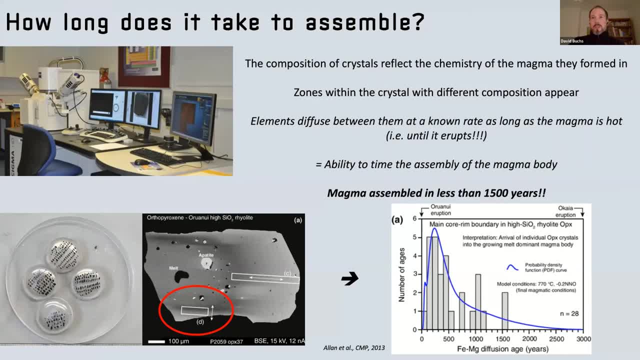 kind of a broad question. So you mentioned that a lot of the eruptions that took place over the last you know few thousand years in New Zealand were really really big and that the volume of magma that was associated with this eruption was also extremely big. And then you said: actually it doesn't take. 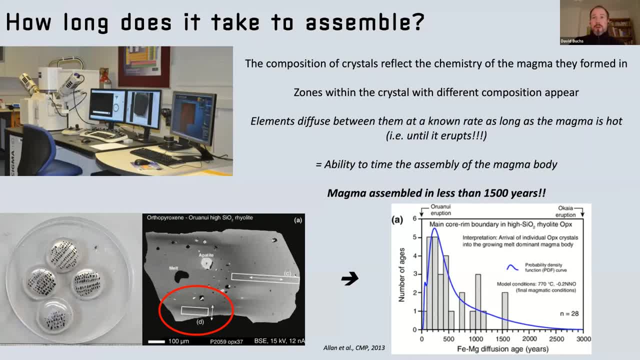 very long to store all that magma before the eruption in the upper part of the Earth's crust. So and you said then that that means you know we could have a major super eruption building up relatively quickly and perhaps we think an area is safe and it might not be safe. 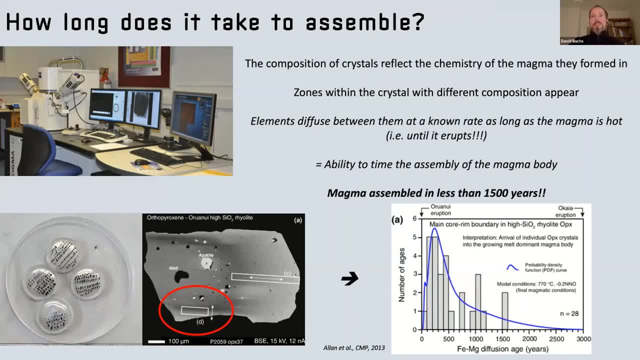 But in that case, because the volume of magma being injected into the crust is so big, wouldn't be able to kind of measure deformation at the surface, especially with modern technologies like GPS? Absolutely we would. I think we would. A geophysis would be a more better place. But 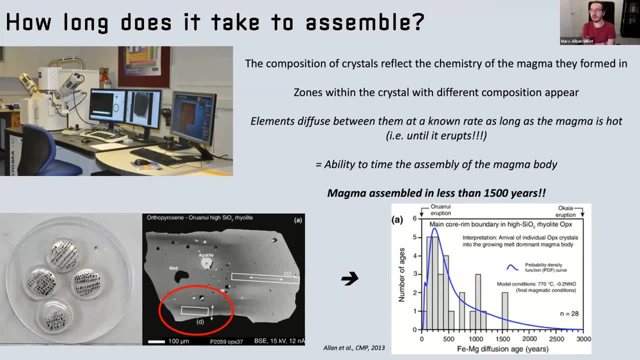 I guess it all depends as well at what depth the magma is stored, And in the case of the tap, the, it is stored somewhere between three and eight kilometers deep. So you know we're talking about injection of something into the crust. Yeah, probably we would be able to. 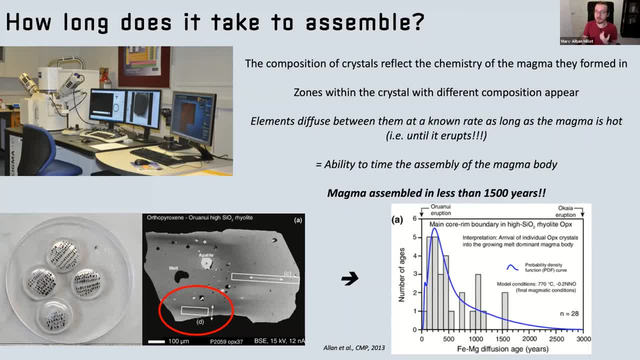 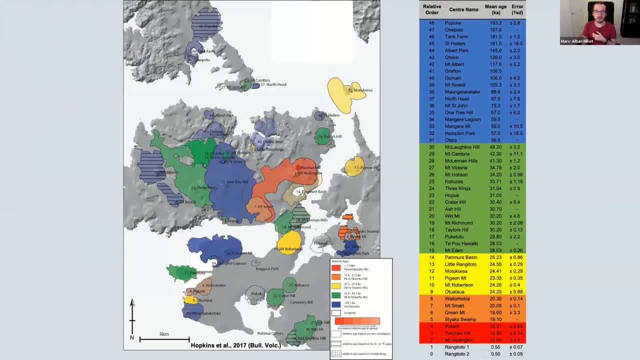 One thing to note as well is that one of the reasons why we have this in New Zealand is that- and I'm just going back to, of course, this is come back to the animation- So it is that this is actually in the rift zone, So we do actually make continuously. 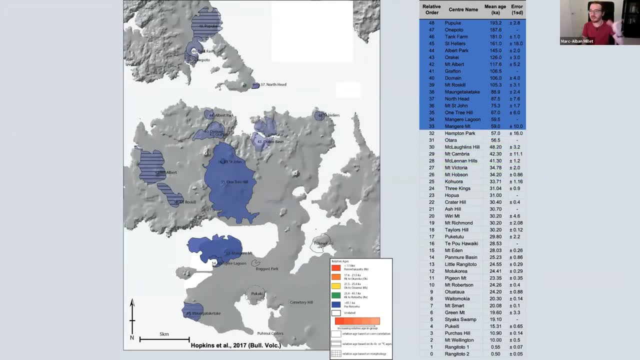 we continuously make room for more magma to accumulate in the shallower levels of the crust, And that is one of the reasons why we have such short timescales for this kind of eruption. So in a way, like New Zealand in the tap volcanic zone is kind of a special case here. 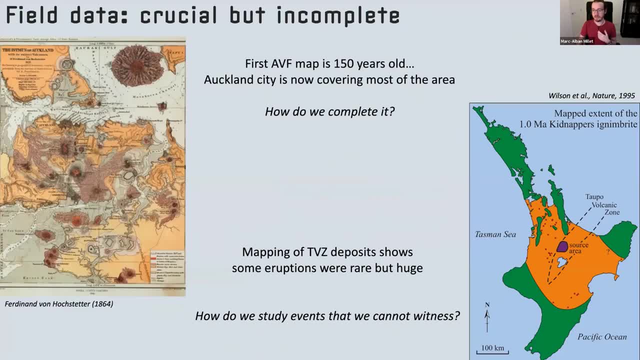 Pardon me, That's there. So yes, Basically this is the type of volcanic zone here, And this is a volcanic zone and a rift zone that is opening this way, So continuously spreads and opening sort of like two needles on. 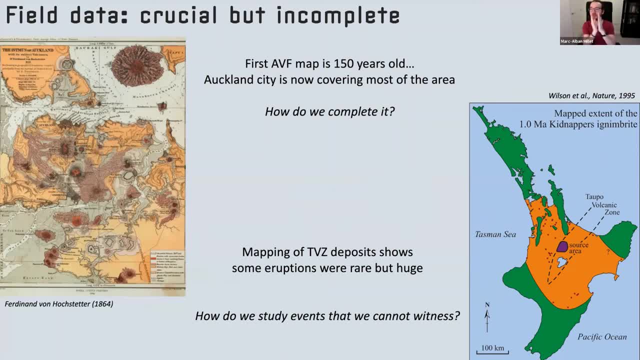 a clock going clockwise, essentially, So you do make this room for more magma to come up. So, yes, I would say yeah, we probably would be able to, at least in the final stages, measure ground deformation. Yeah, Excellent. So that's kind of a reaction. 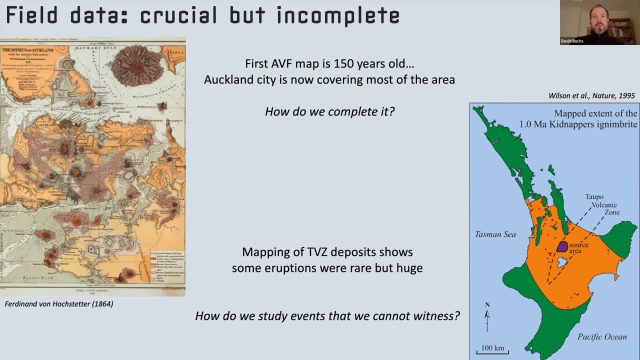 I guess, especially if you live in New Zealand, although they've got so many problems, And actually since then Colin has been working a bit more and now got a big project and actually trying to nail that a bit more. It's called Eclipse And with many PhD students and postdocs, 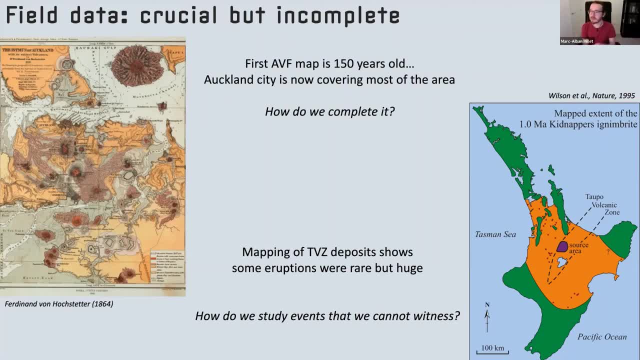 working on the more you know responsive and aspect of things. Yeah, Interesting, Great. Yeah, There's another question. Each volcano has a distinctive chemical signature, So the magma has a different composition. Doesn't this evolve over time with possible? 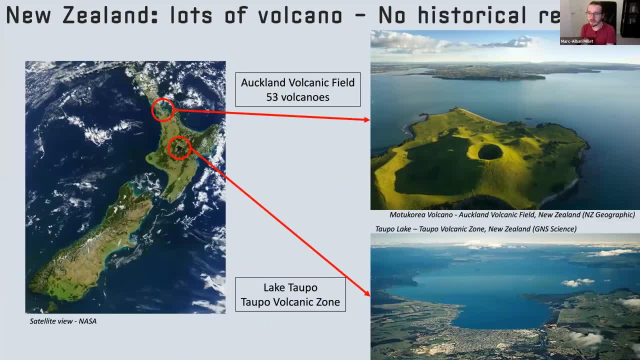 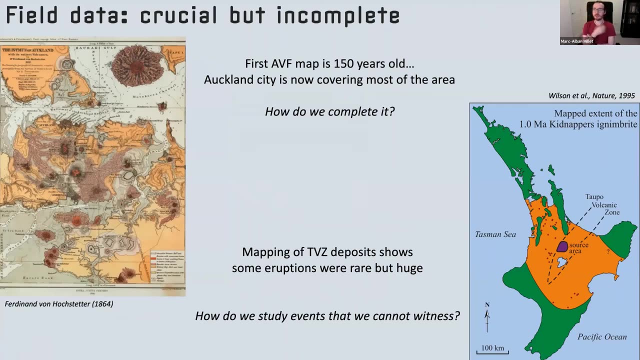 confusion as a result. That is correct in most volcanoes In Auckland. the main thing is that we know that each volcano only erupted once, So that is really helpful in that regard. So you know they have this composition. We know that this ash erupted and that's it. after that magma never came. 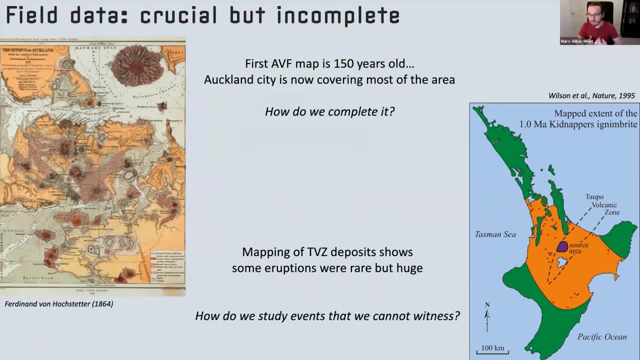 back And this is what we call a monogenetic volcanic field. So yeah, so essentially we. you know, the difficulty there is that if we were only taking one single sample out of this volcano, just taking the rock that is the easiest to find from the compound, for example, 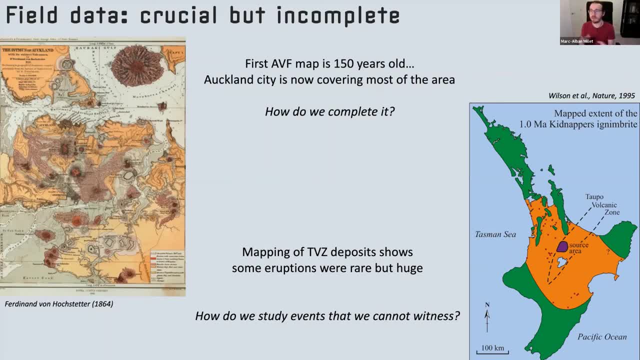 we would be underestimating the viability within that volcano. So each of these we have, you know, sample 10, 15, 20 samples, sometimes depending on how big the volcano is, to have a good idea of the range of composition present in that volcano. 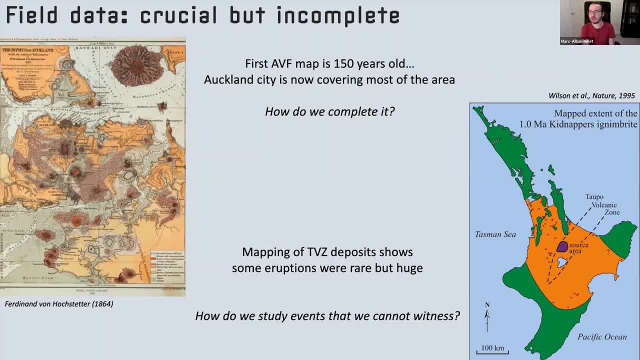 But you know the fact that actually these volcanoes only erupted once, you know, or were active in one go and after that died out was pretty handy to do that work And that's why this method works there but may not be applicable in the. 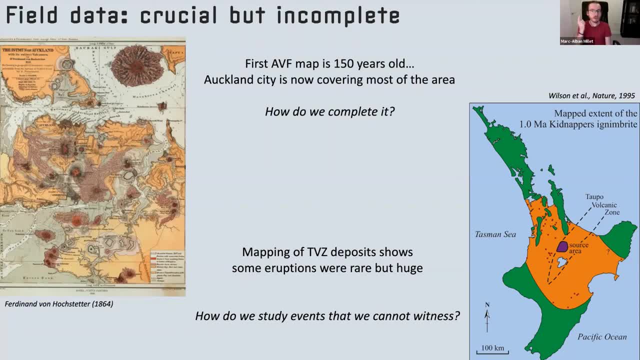 exactly the same way everywhere else. So so, yeah, that is the reason why- but that's also part of the danger in Auckland is that we know that if magma comes back, it's going to come back somewhere it hasn't erupted before And we need to find out where. So yeah, so that's, that's. 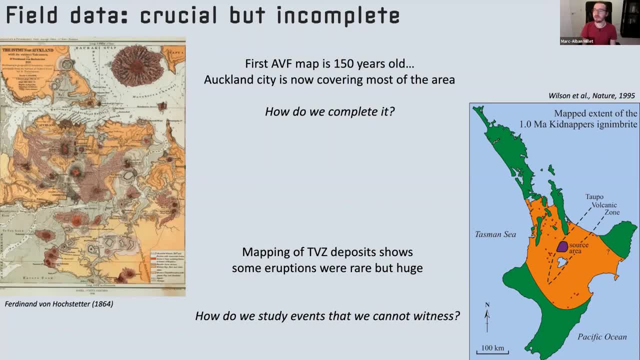 parts and parcels of you know, studying a monogenetic volcanic field like Auckland. Oh great, So there is no other question in the Q&A panel, but I might ask a final question. So I think it's interesting as general principle or idea you mentioned that we can. 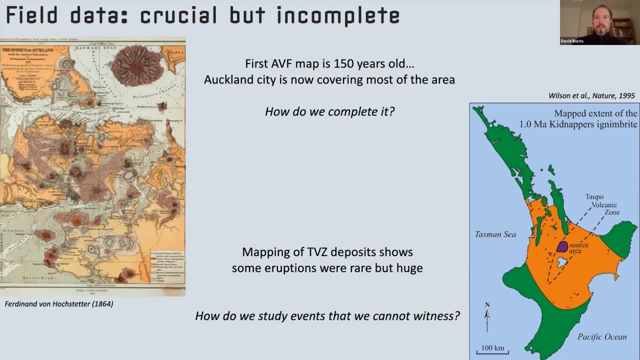 constrain or calculate the pressure of emplacement of the magma. How do we do this? So what we do again is actually: the chemical composition of the crystals are dependent on many variables, So you know when. so that happens, that you have the chemical position of the magma. 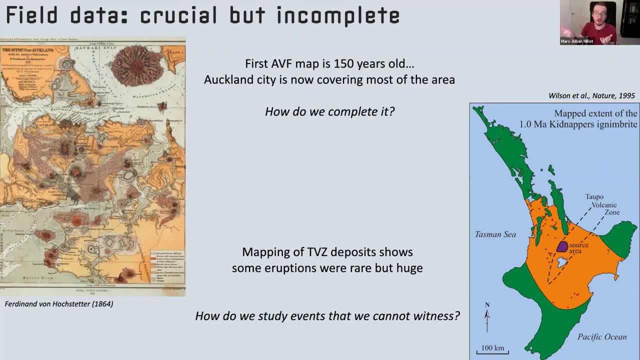 the temperature and the magma, And then you have the chemical composition of the magma And then- and the pressure will affect the chemical composition of the crystals being formed in slightly different ways And some crystals actually are going to be different. I'm only responding to these different parameters in different ways. So some elements as well.